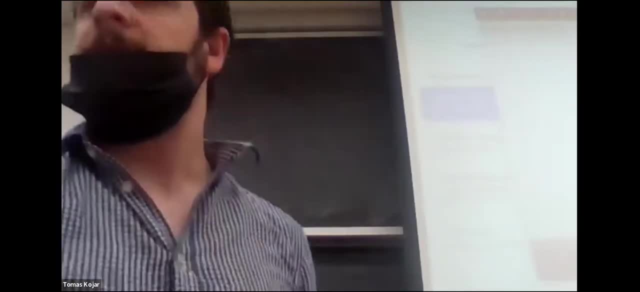 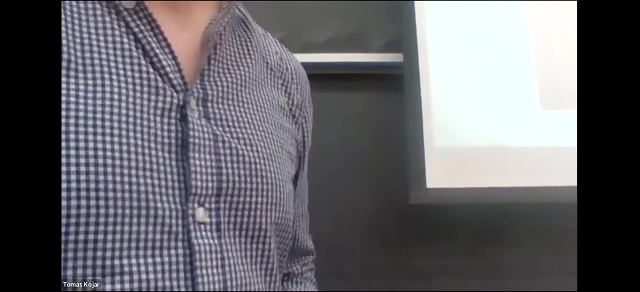 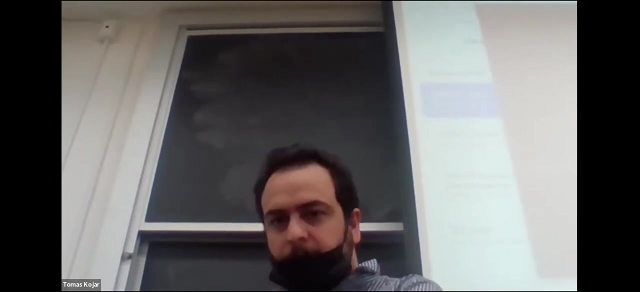 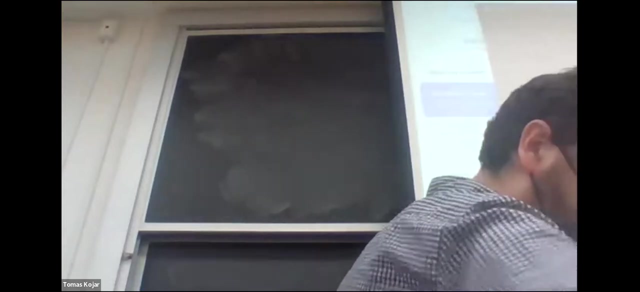 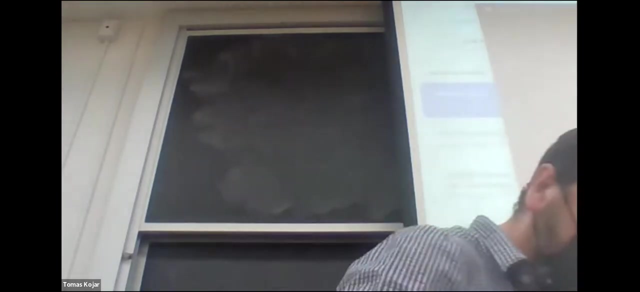 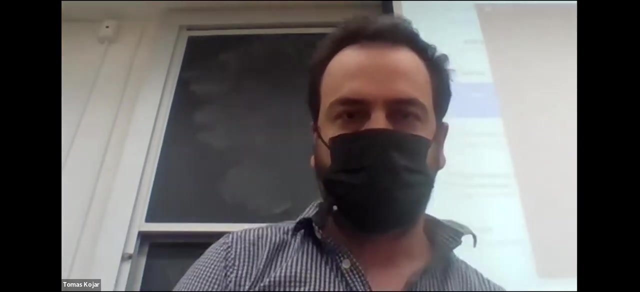 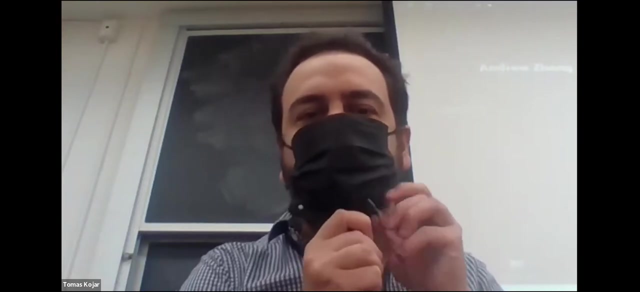 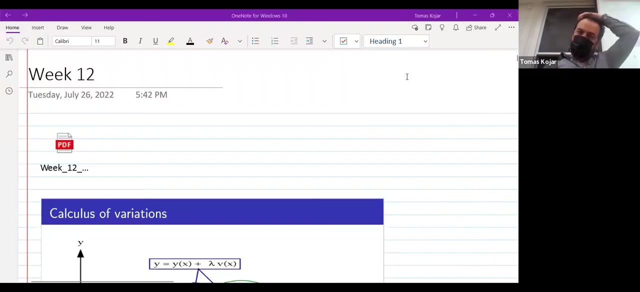 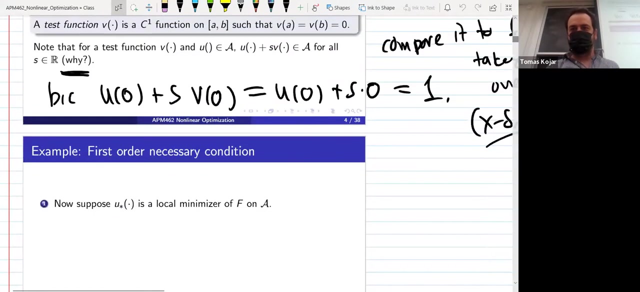 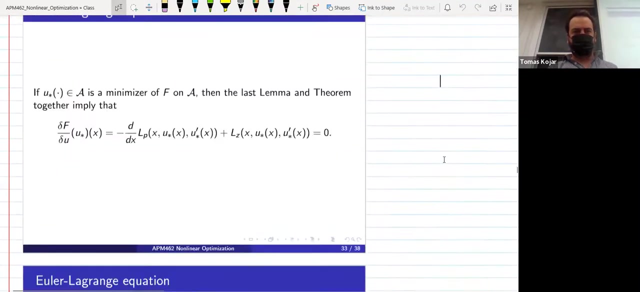 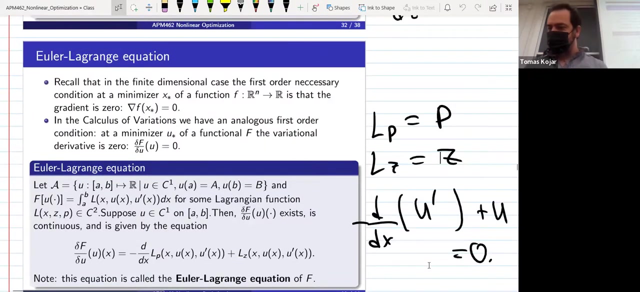 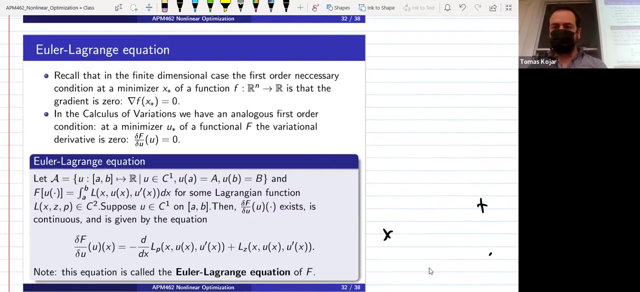 Thank you, Can you hear me? Okay, All right, Any questions? Anybody? No, All right, All right, Good, Let's start. So in the homework, right, you have a bunch of functionals like this guy. 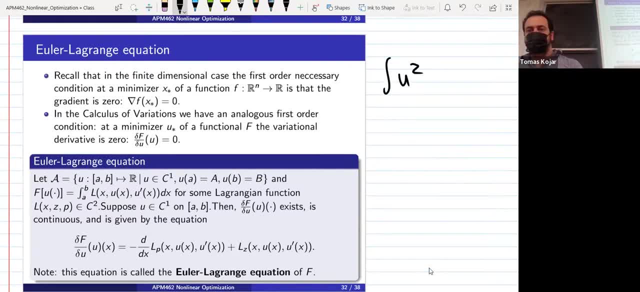 So like u squared and u prime squared, And the question is to find the Euler-Lagrange equation. So let me do this one. We'll do a bunch of examples And I ask you to do part A and B. So do all the parts the easy way, okay, which I'll do now. 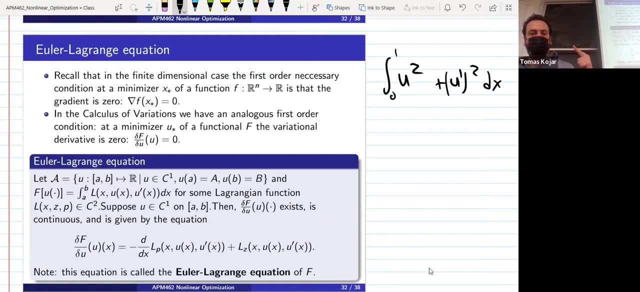 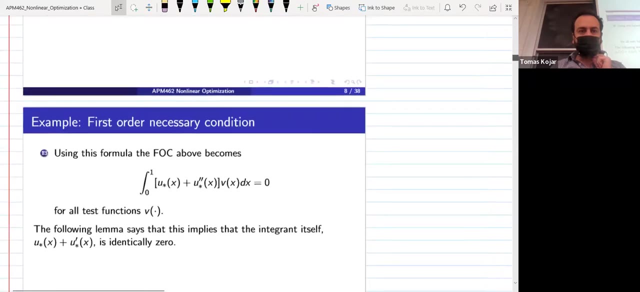 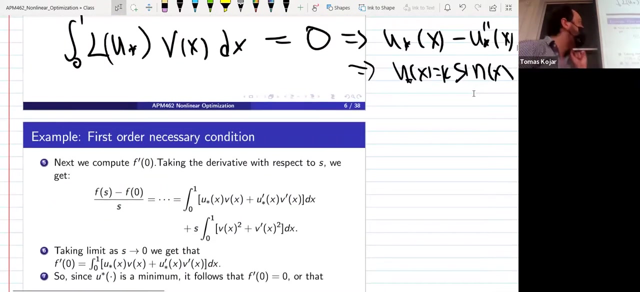 But then do just parts A and B A little bit harder, just to understand what's going on at the back. I want you to take the fractional, the variational derivative, like I did in, And yeah, so I want you to do this guy. 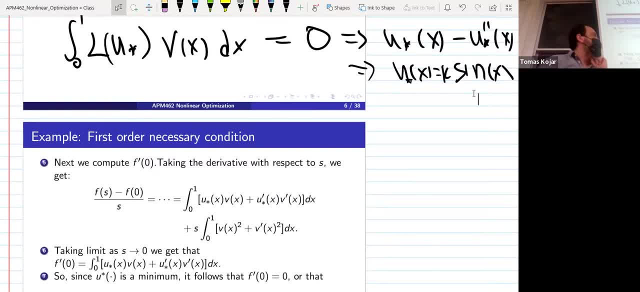 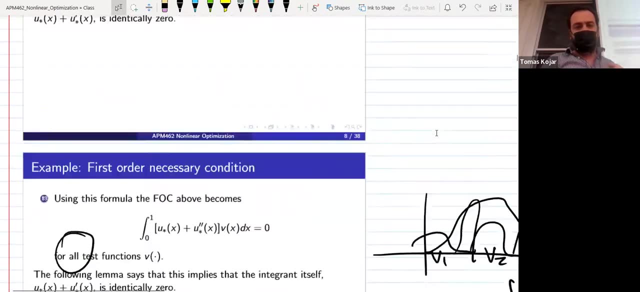 For parts A and B. okay, All right, You'll see when you get there. Anyways, this is for next week's stuff. Yeah, so that's what we did last time, But now I'm just going to use the result to get the same ODE. 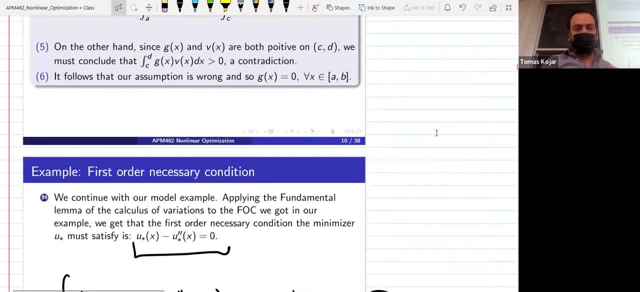 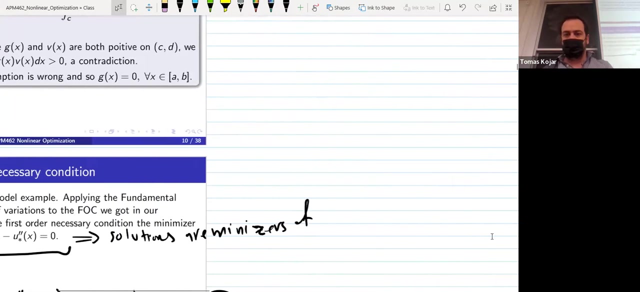 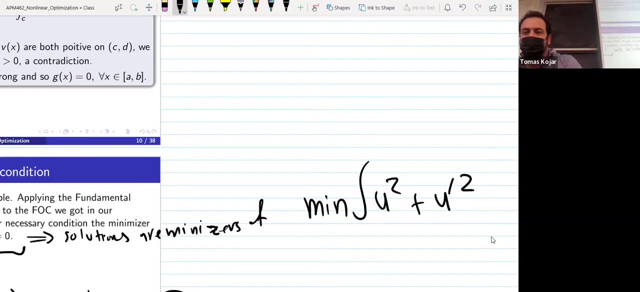 So we got an ODE last time over here We got this ODE, meaning that the minimizers, the solution, the use of this guy, are minimizers of the following: optimization problem: Min of the functional u squared u prime squared over all u with u zero, u one equal to one. 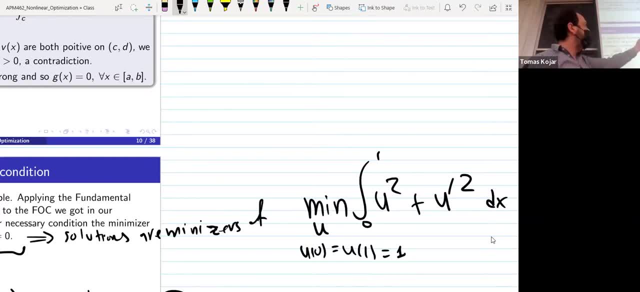 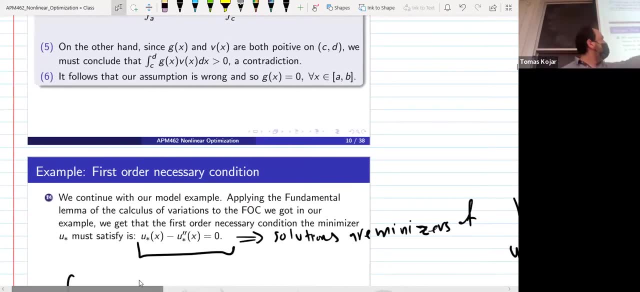 Is that okay? Okay, good, So this is a minimization problem, And I will prove today a theorem that says that the minimizers are always given by an ODE, which is called Euler-Lagrange. Okay, All right, So let's do that. 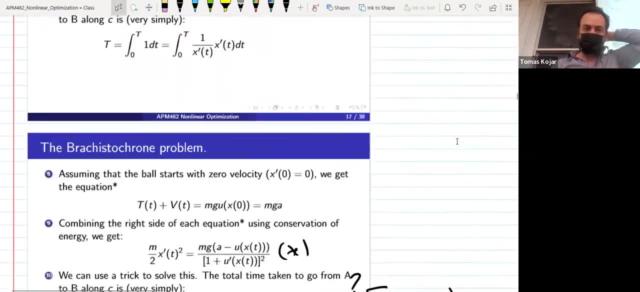 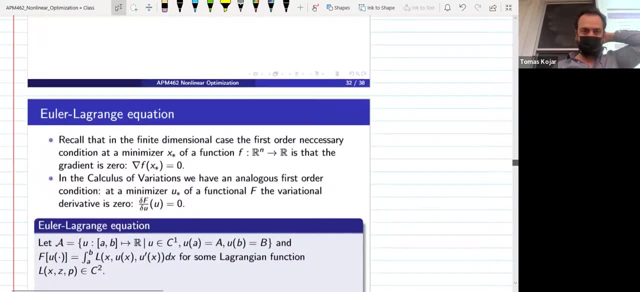 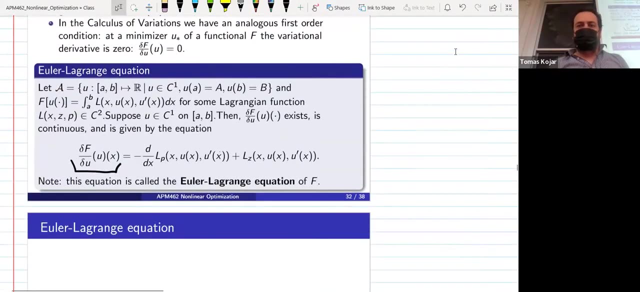 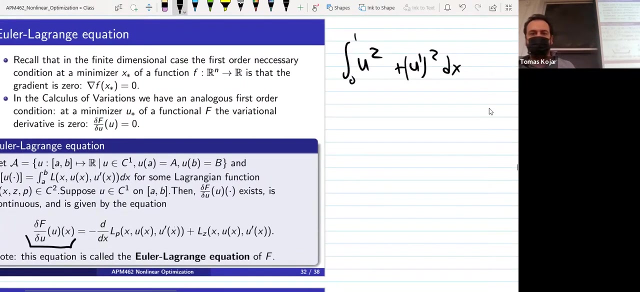 Let me do the. let me show you how to apply the theorem. So let's do it for this case, just to see if you understand. Can someone tell me what is LZP? Sorry, LXZP for this functional. Any ideas? 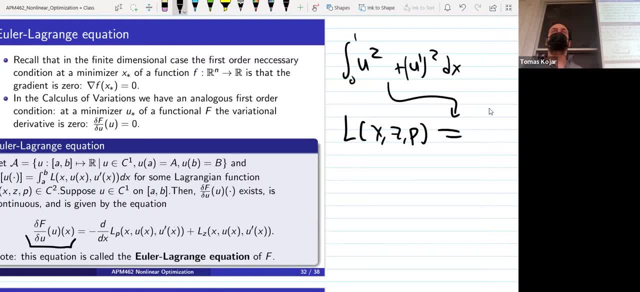 Whatever Here, or Zoom, Zoom people, do you know? huh, What? Yeah, So Zoom, do you know, Andrew? Yes, thank you, Michael. Good, No, no, no, there's no X. No, because you have to match the variables right. 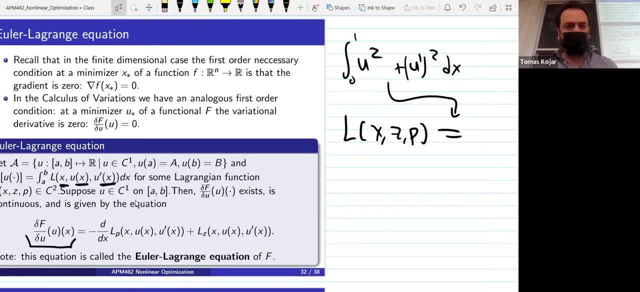 Okay. So, Michael, yes, perfect, All right. And then you, you take this derivative, So let's do it. So first we take L, partials Z, which is you said it was, yeah, what is it? 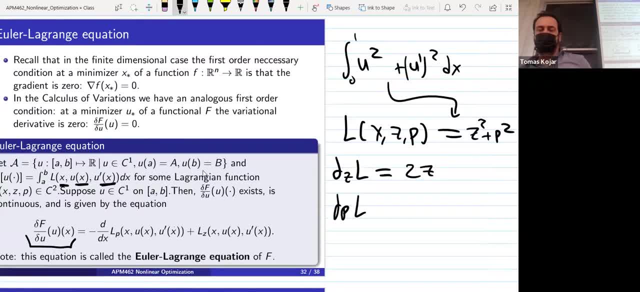 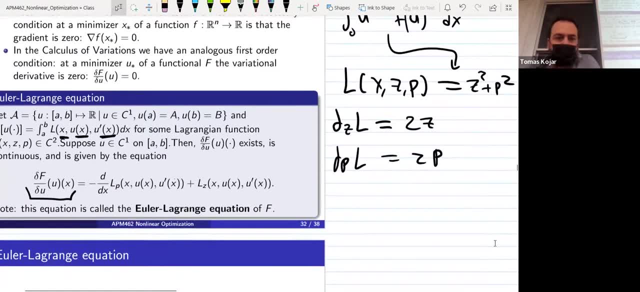 Yeah, And partial of P, And now let's find the ODE. So So, Okay, Okay, Okay. So you plug in Z equal to U. Okay, So you plug in Z equal U and P equal U prime. Okay. 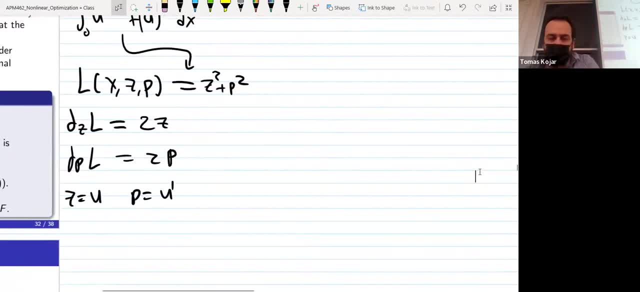 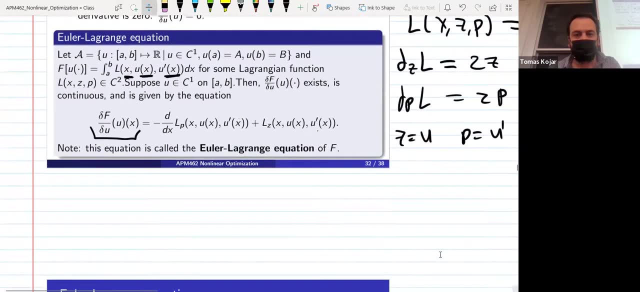 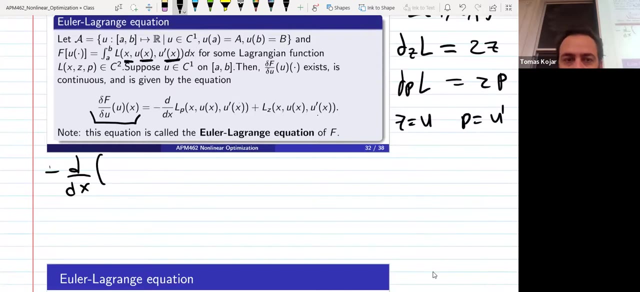 So now, Okay, I want to have it on one page, All right. So I have minus DDX of L P, so two P evaluated at P equal. what, Yeah, you prime X plus um two Z evaluated at Z equal. 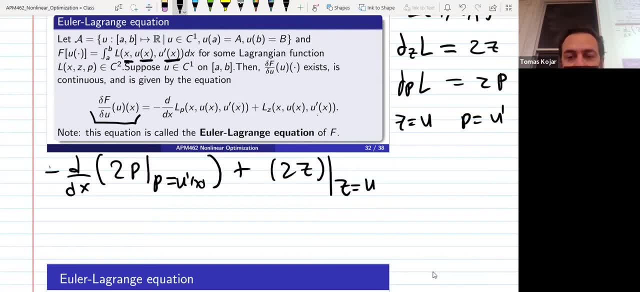 Yeah, and you set this guy to zero, Remember, is that okay, All right. So So the first guy is minus DDX of U prime X, and this guy is equal with a two and then a two times a U of X. 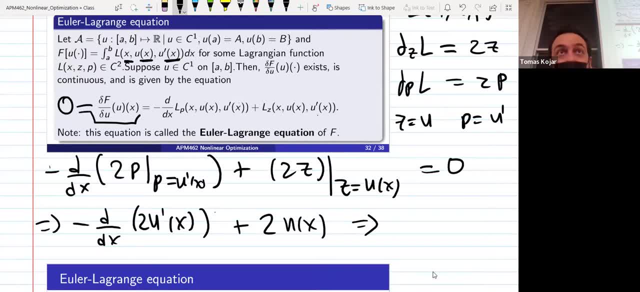 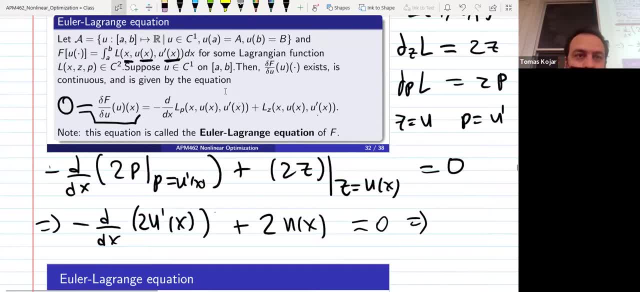 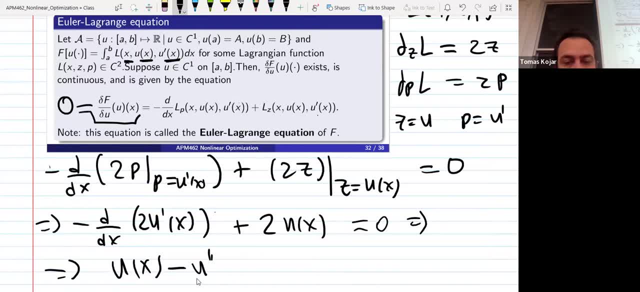 Yeah, Okay. So that's all I want you to do for question 15, the homework For all the parts, But for parts A and B I want you to do what I did with the variation. Okay, Okay, good. 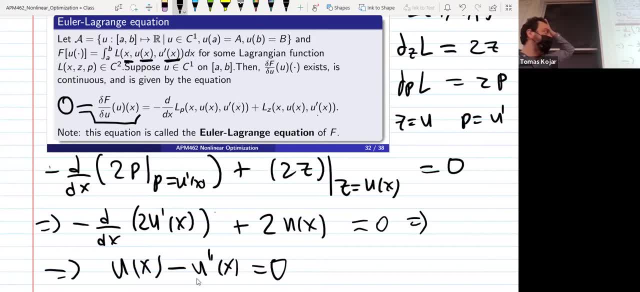 Everybody happy, All right. Thank you, Bye-bye, Thanks everyone, Bye-bye, Bye-bye, Bye-bye, Bye-bye, Bye-bye, Bye-bye, Bye-bye, See you, Bye-bye. 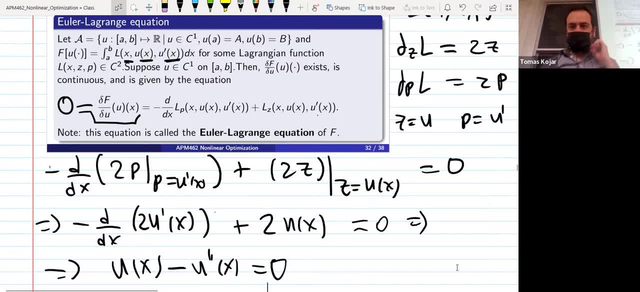 Bye-bye, Bye-bye, Bye-bye, Bye-bye. So now I'm going to prove this so you don't have to move it besides parts A and B. So you can just use this. but this is always given by this early Lagrange, the minimizer. 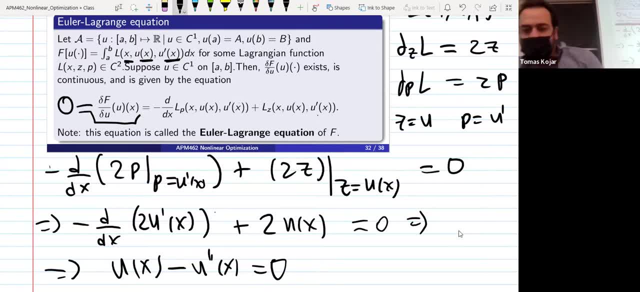 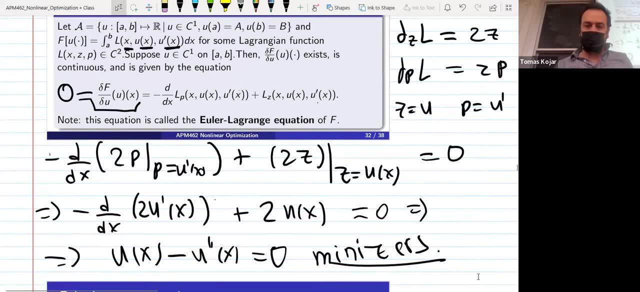 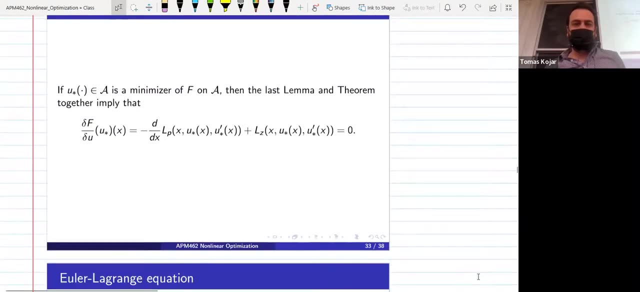 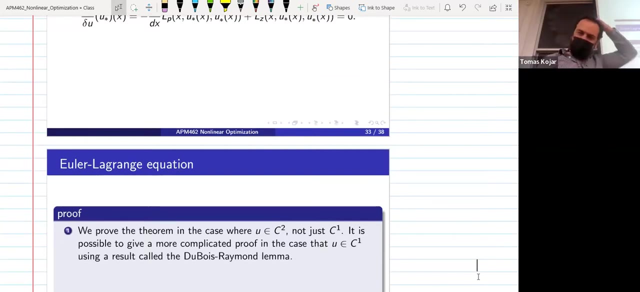 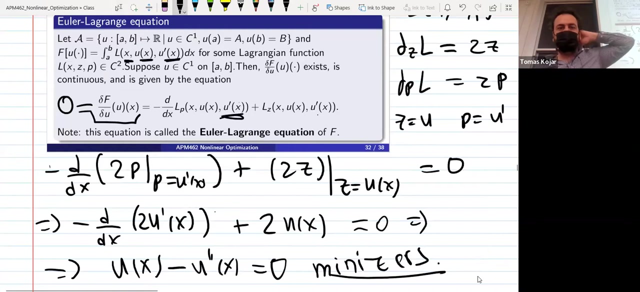 So these guys give you the minimizers. So this is minimizers. Okay, let's go. Yeah, so if this guy is there, yes, equal to zero, yeah, okay, good. So yeah, I have to assume C2, because here you take, you have one derivative inside the 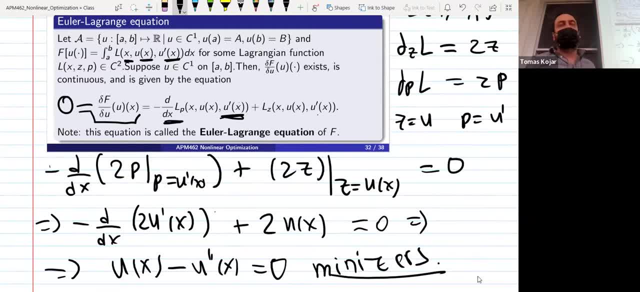 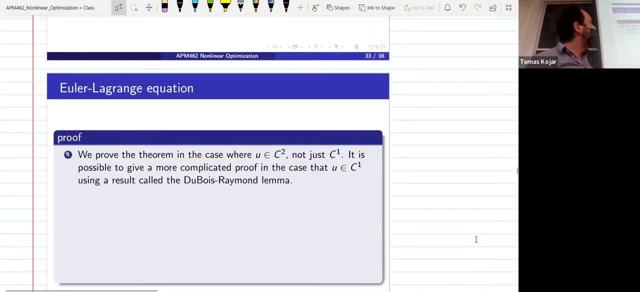 Lagrangian and you have another derivative outside, So you have to take a double derivative, okay. So that's why I assume, Okay, So I assume that the guy has two derivatives, C2, and yeah, whatever, you can relax it. 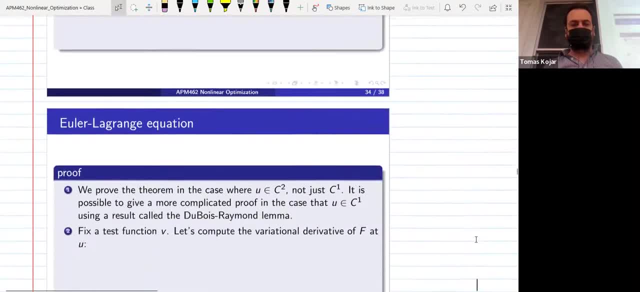 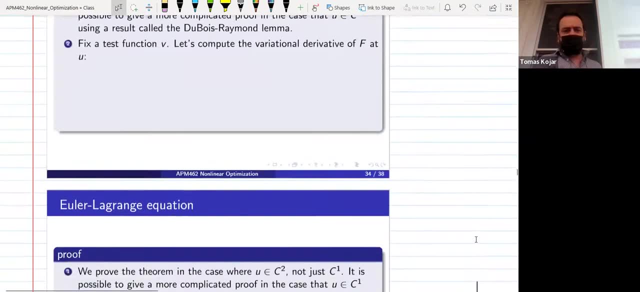 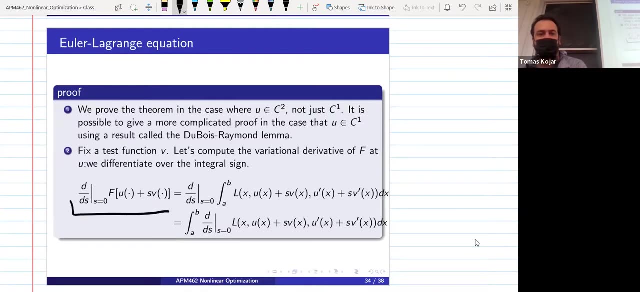 We're not going to go into that. So what do I have to do? Well, remember what is variational derivative. oh, I jumped too much. Variational derivative was this guy over here. So we, we. this is the directional derivative. 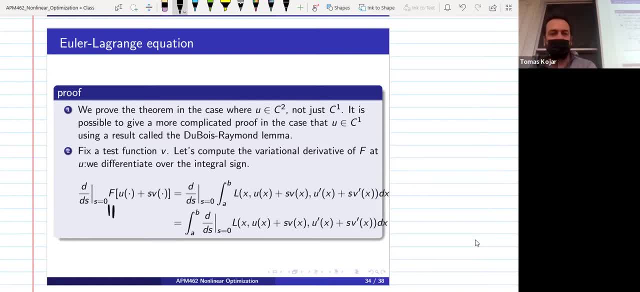 And remember, we have this formula that this guy is equal to a, a, b, and then you have your g of x, and then you have vx, right, And then we call this gx to be the variational derivative. Okay, 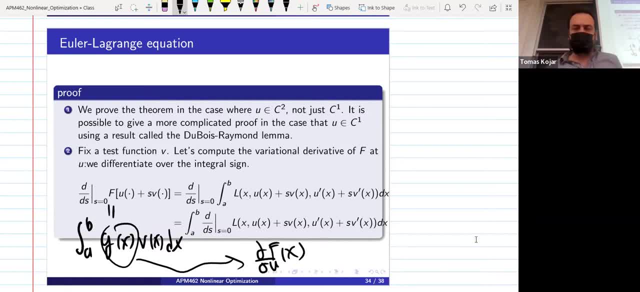 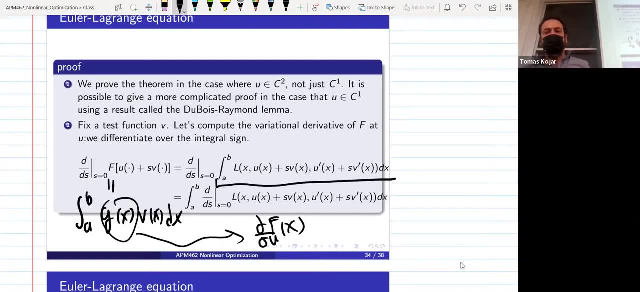 Okay, So, yeah. so this is a bit of a long proof. It goes step by step. So my definition of my function will always be of this form. Okay, It will always be like this. And what did I do? I subbed in my perturbations. 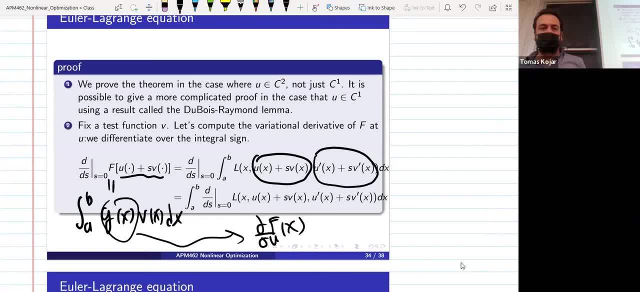 Okay, So I put in my perturbation over here, So perturbation. And in the next step, which is called refinement, it has many names, but it called Leibniz, derivative under integral. Okay, We did this in analysis. 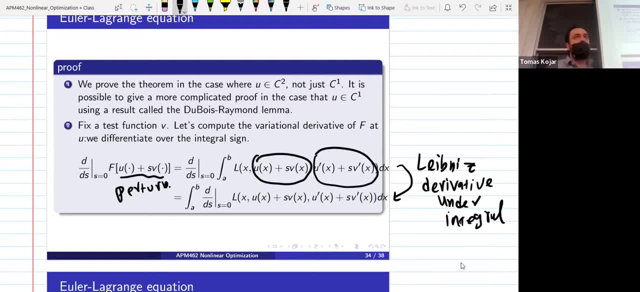 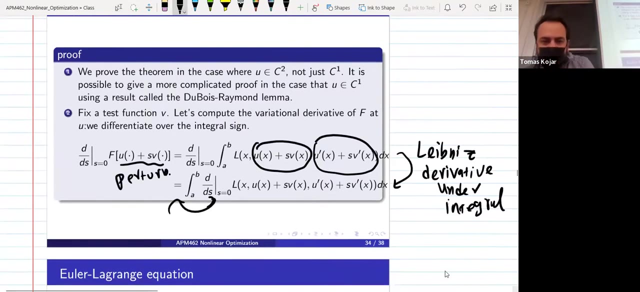 but it requires quite a bit of justification to be able to swap. You see, we swapped the two right And that's not obvious at all And it's beyond our course. You're welcome to come to analysis. Yeah, Okay. 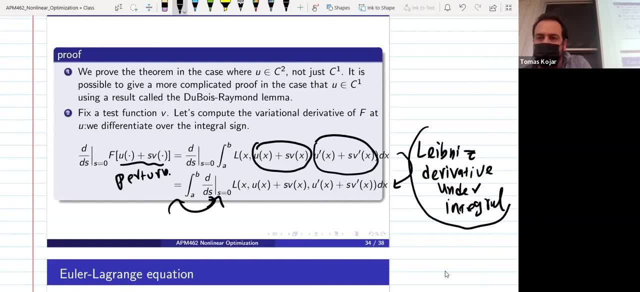 I mean I'll write the name It's called. yeah, it's the one I just called here: Leibniz differentiation under the integral. Okay, So if you want to look it up and understand what happened, look up this thing. 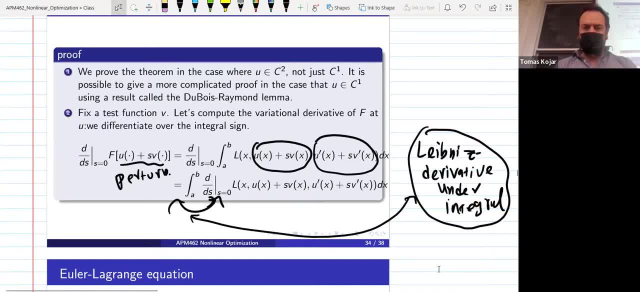 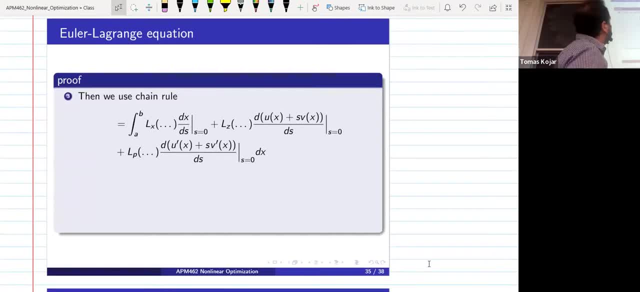 It's a theorem, All right. So you do that. I mean, oh no, it is ugly. Yeah, Then what did I do here, Any? I mean, I did chain rule, sure, But this is called also a total derivative. 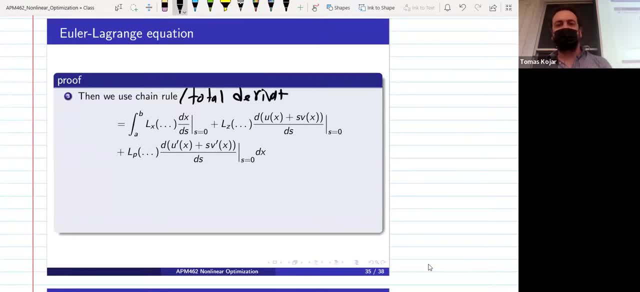 We did this in office hours and it took us like 20 minutes. So you have whenever you have a function. so you have a function of three variables here: L? L of X, U L of X And plus SBX, and then U prime, SB prime. 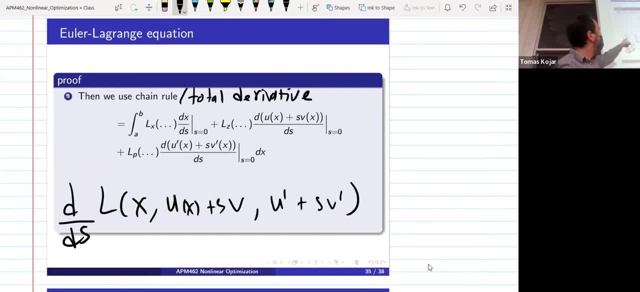 Then when you take DDS, you have to take DDS of each variable, right? So I do it the first guy, I do the second component and I do the third. Okay, Is that okay, All right, But then X is just a variable. 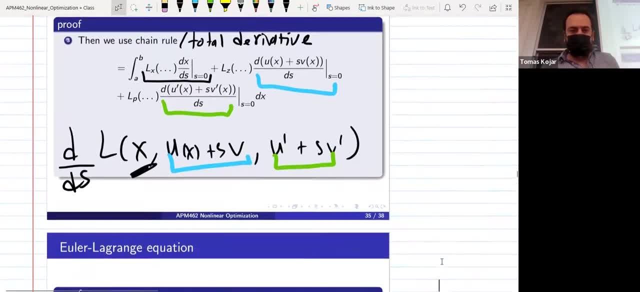 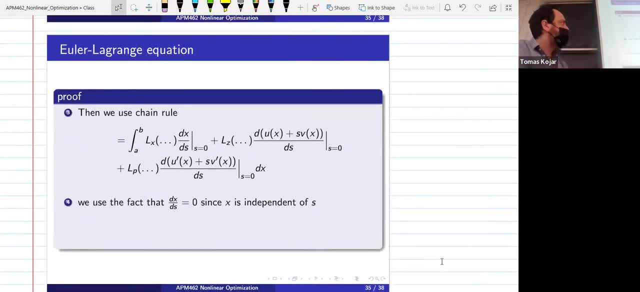 I mean, it doesn't depend on S, So it's zero, So that guy's out, That guy's dead, And so you're left with this two, And let's see Where am I. Okay, Okay, Okay, Okay. 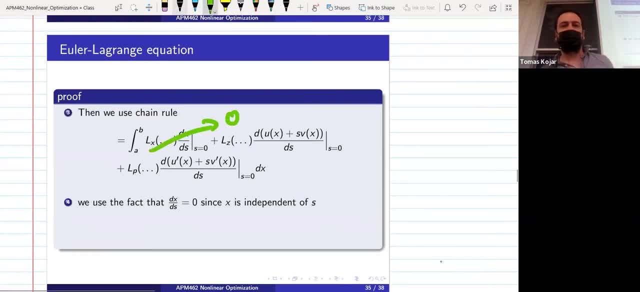 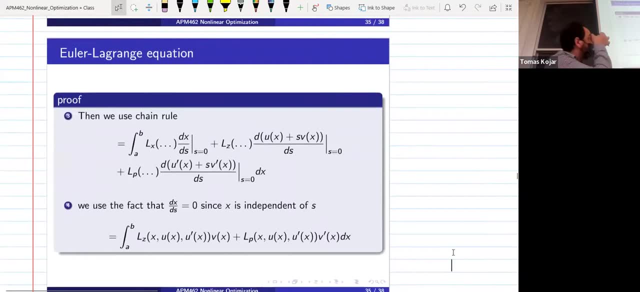 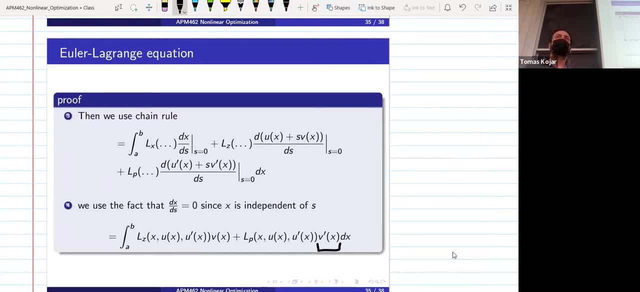 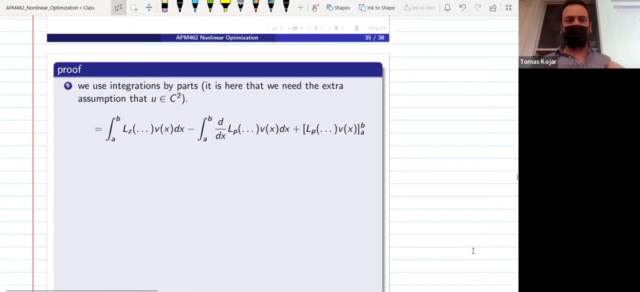 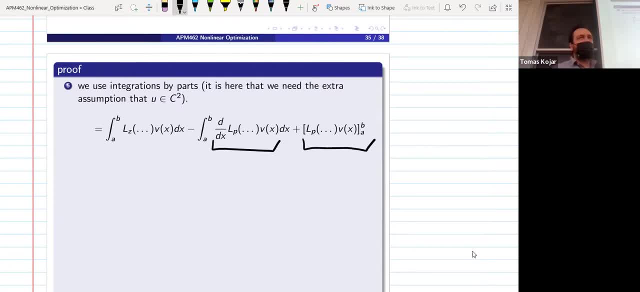 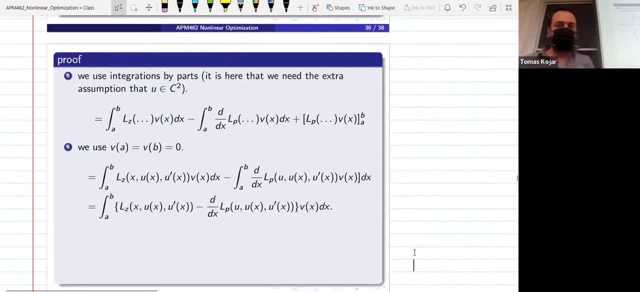 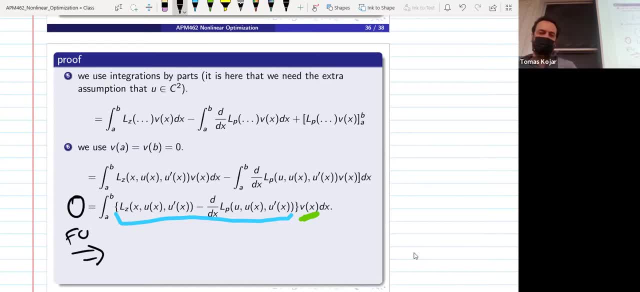 thing, yeah, foc, it stands for fundamental. what do you think the? what do you think the o is? it's like jeopardy. fill in the blank: what's oh, off, and then what's the c? yeah, yeah. so again, just to remind you the result, because i want you at least, at least know that. 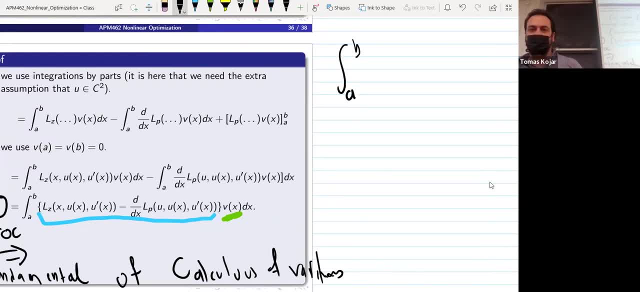 if you're gonna do this. yeah, so whenever you have some function, call it g of x and you know that this is always zero for all test functions, so for all guys that satisfy that, satisfy this, then g of x is identically zero. okay, so we did this with this epsilon delta argument. 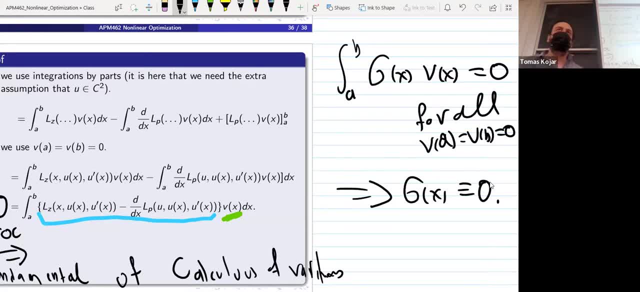 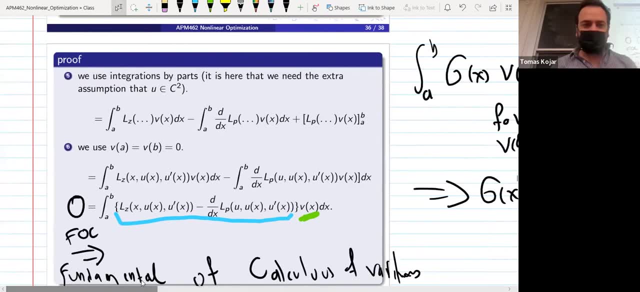 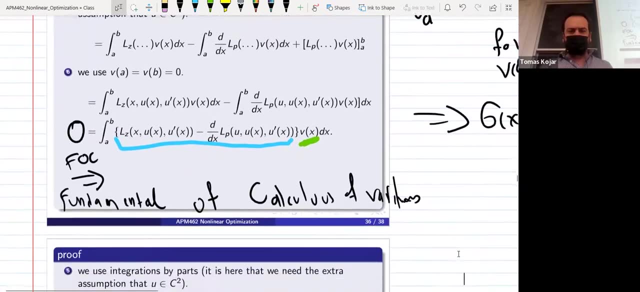 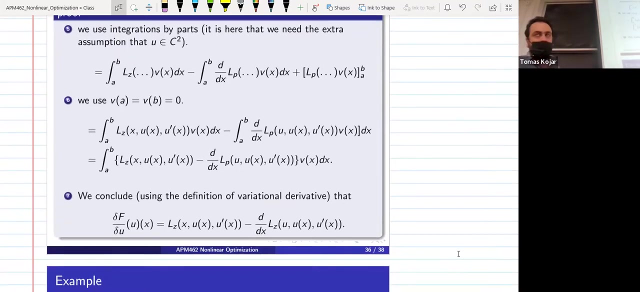 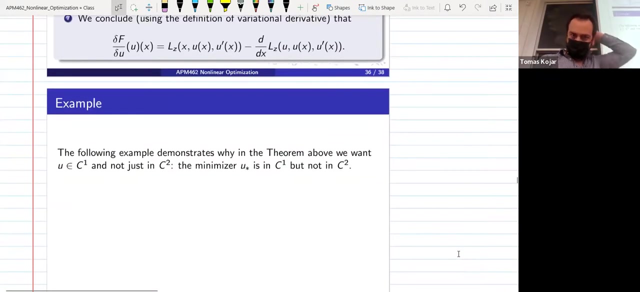 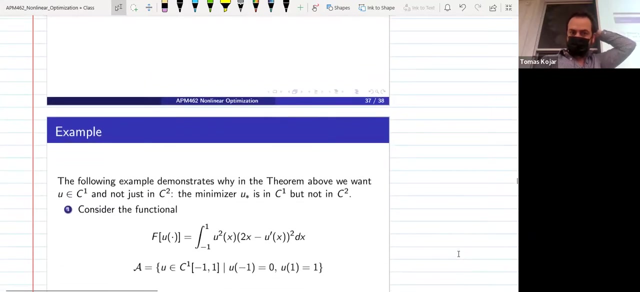 which you call it lambda, lambda, epsilon, yeah, no, epsilon lambda. that was your yes, good, all right, any questions? that's really the main result and uh, okay, so yeah, and that was our definition of the uh variational derivative and we'll let this go, so that i thought it was quite simple. 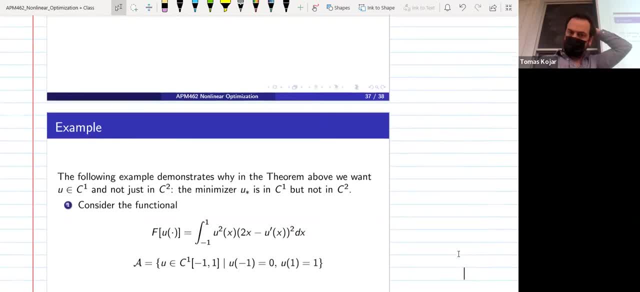 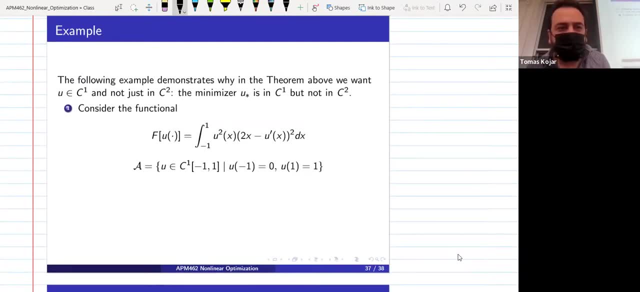 so, but anyways, i think i mixed up the. i think i mixed up the. uh, this should be the other way around. makes no sense. that's weird. okay, so i forget. what was the next one. number two: Right, so now let's do an example, just to you know, get some practice. 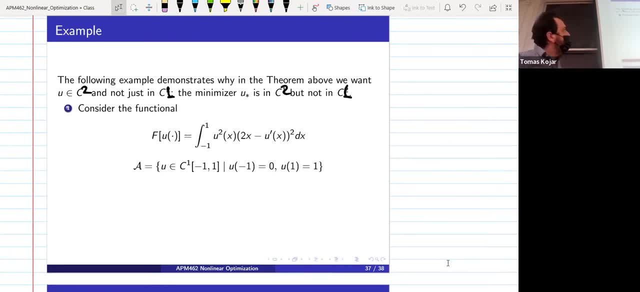 So here's the functional and you'll see that it's minimizer. If I remember correctly, it's not C1.. I probably have it, Okay. whatever, We'll see what I don't remember now. Yeah, this is my functional. 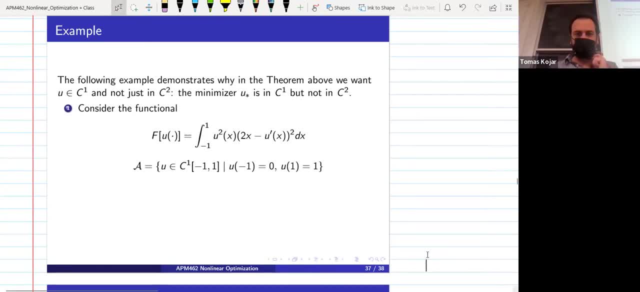 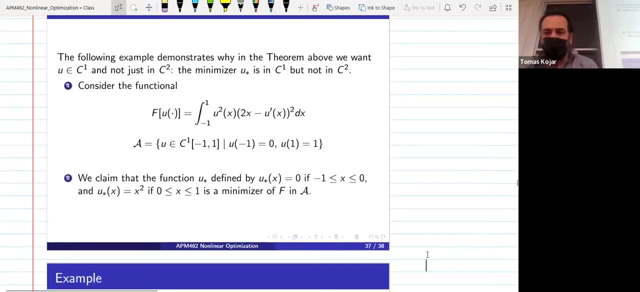 and I'm going to give you the Euler Lagrange. Yeah, let me draw the function. I mean, I want to find the equation first. Guys, let's find the equation first. Yeah, let's just do that, guys, It's more fun. 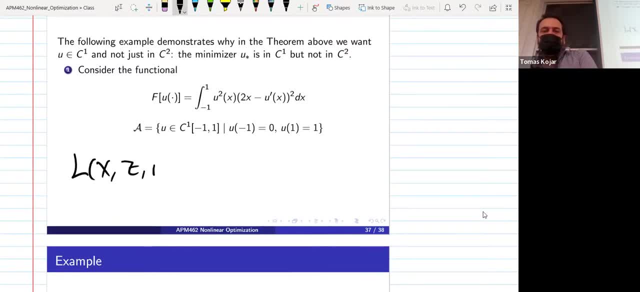 So can someone tell me what is LXZP equal to? What's the Lagrange? Zoom people and hear people Zoom people. What do you think? What is it? Yeah, Z squared Good. Was that Michael? Oh, no, Andrew. 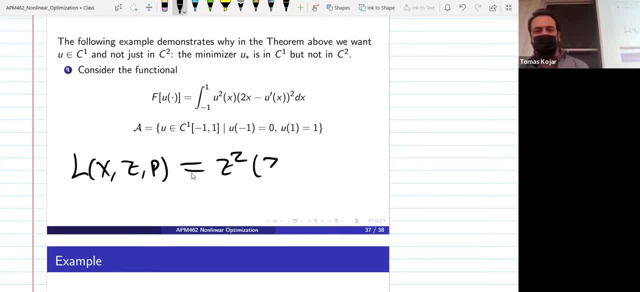 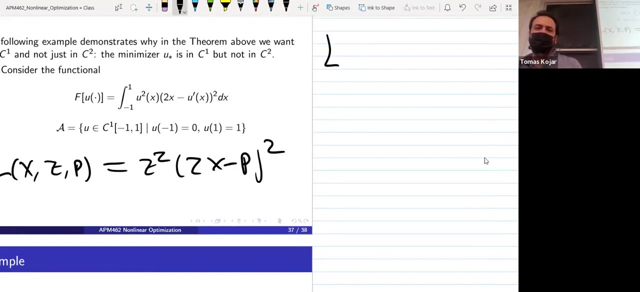 Good job, Andrew. Yeah, Z squared, 2X minus P, All things squared, All right. now let's find the Euler Lagrange. What is L of Z? Or yeah, that's how they write it, But they want to say partial Z of L. 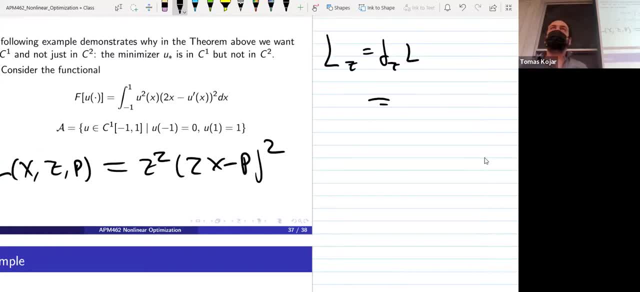 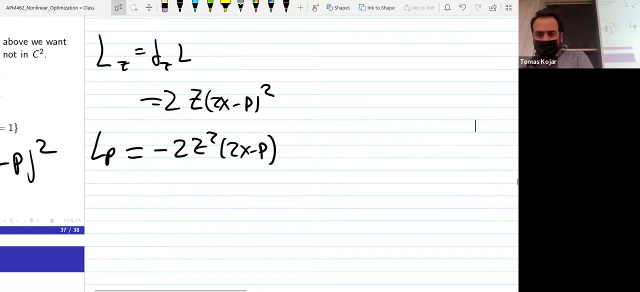 What do you think is the? what is the? Yeah. And then what about LP? Yeah, so as this, yeah, let me put it outside Huh, Good, Now, what do I want? Yeah, so My, my Euler Lagrange, is DDX of L's. uh, no, I want to memorize this. 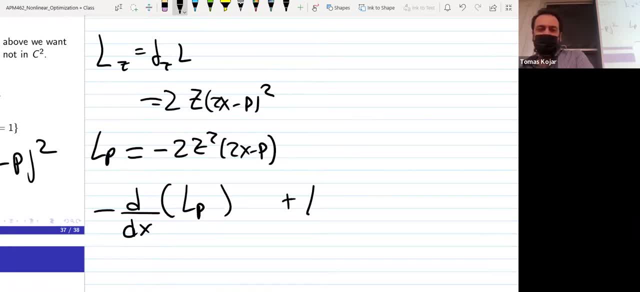 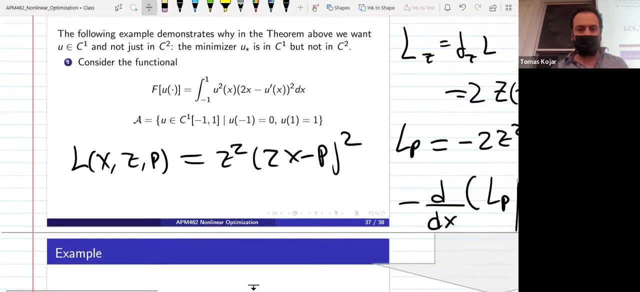 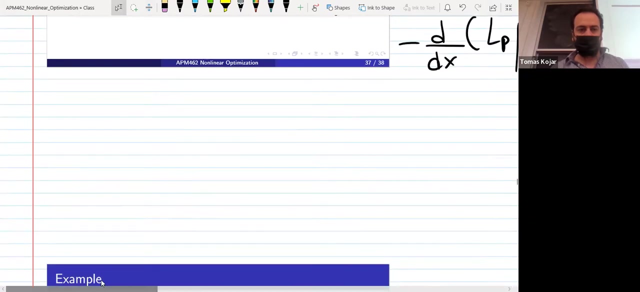 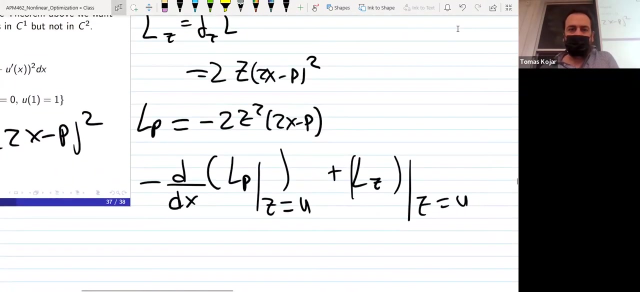 What did we do with? the last guy was yes, And then L of Z. now, and I plug in um Z equal to what, Yeah, And P equal to yeah, Yeah, Okay, I want more space, All right, Anyways. so, uh, okay, let's go. 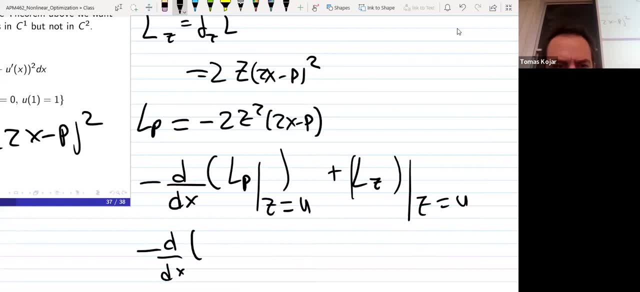 Um, mine is DDI, Okay, So uh, L of X of uh, what Two times? Okay, good, I think you're getting it now, So then it's um, oh, but there's a minus right. 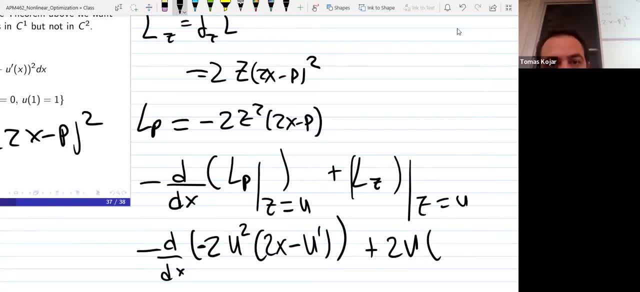 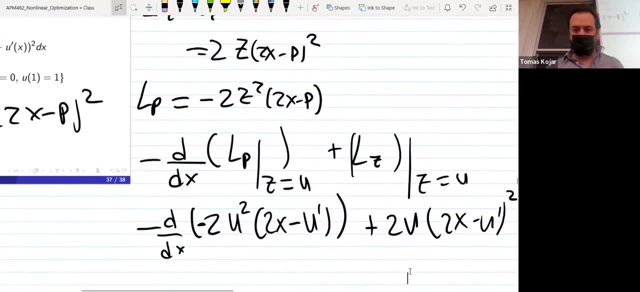 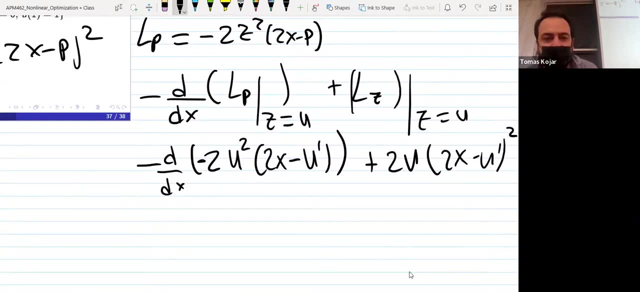 And then, uh, LZ is 2U, uh, 2X minus U prime. All right, I mean it looks terrible. Uh, I don't know. I mean, yeah, that's the idea, I don't know if I I want to simplify it, but at least the minus is not there. 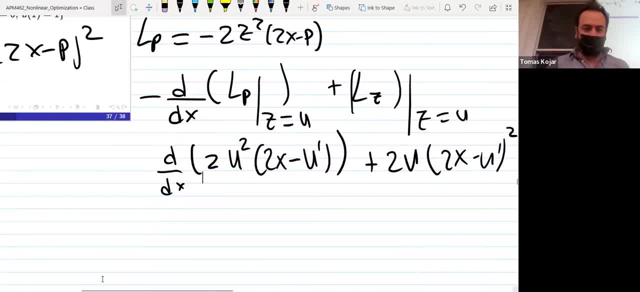 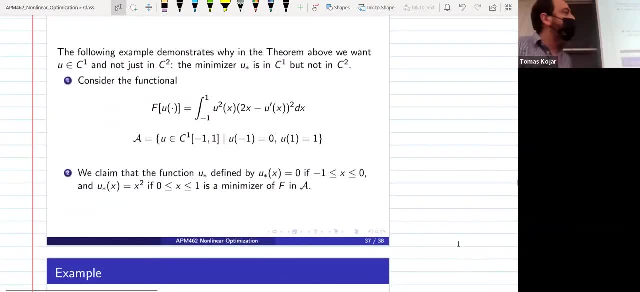 So they kill out. Did I get this right? Okay, We'll check in a second. Uh, yeah, And the? the claim is that the minimizer, the solutions of that ODE, are given by functions that look like this. So it's flat. 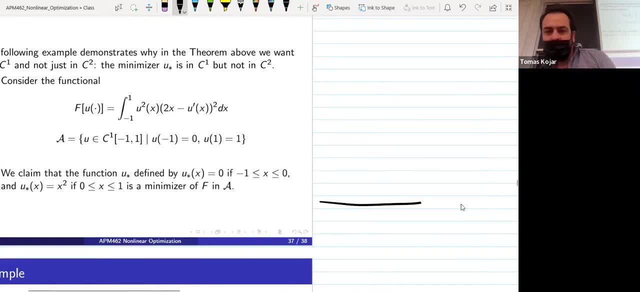 And then it goes like this: All right, Okay, All right, Let's go. Did I get the? yeah, So this is the one. we get that, and the minus: Good, Okay, So, let's go. Okay, So let's go. 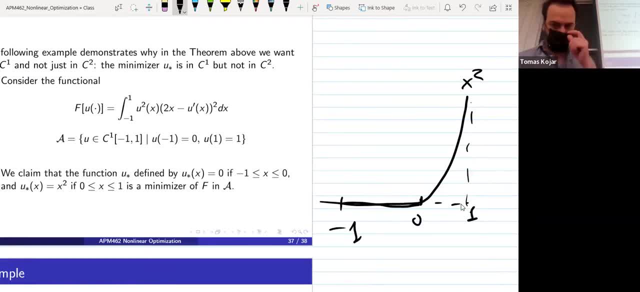 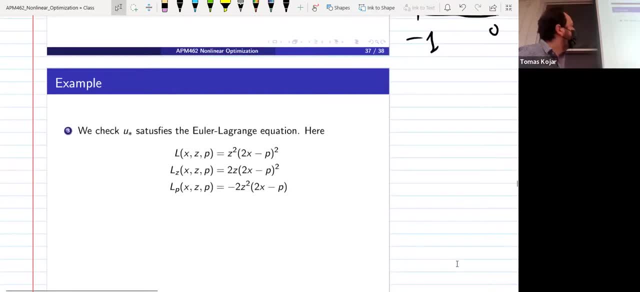 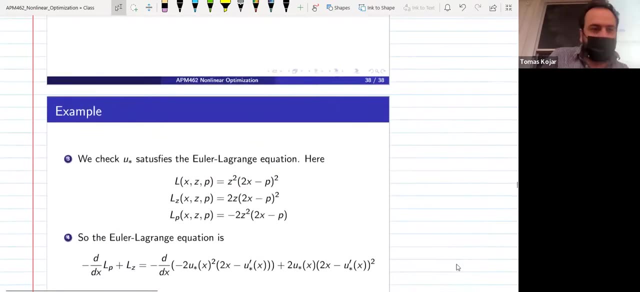 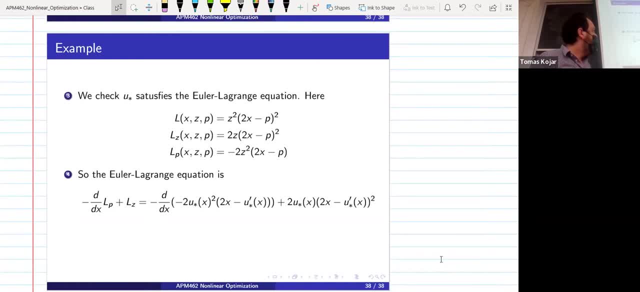 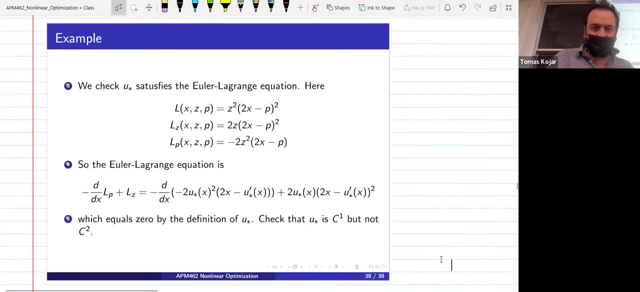 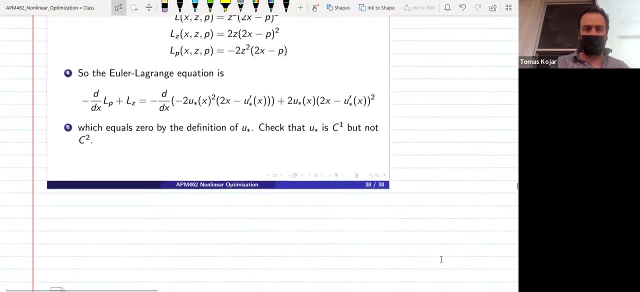 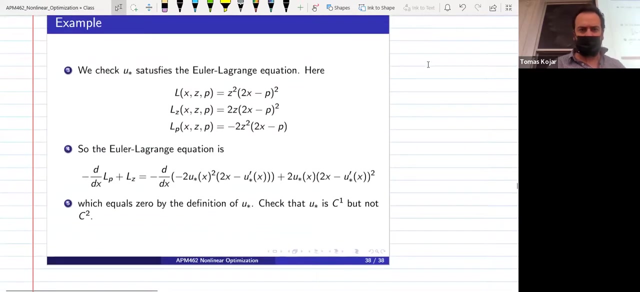 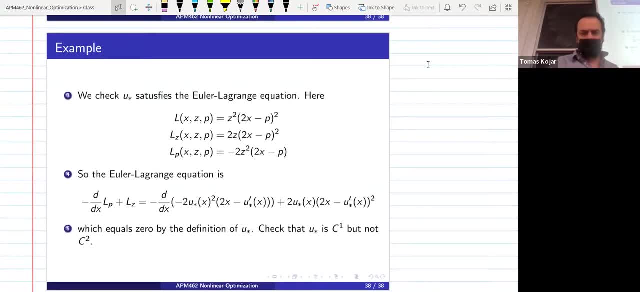 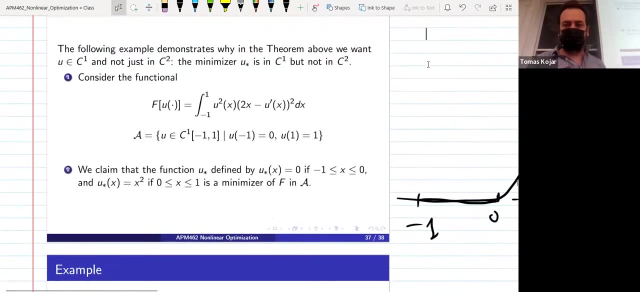 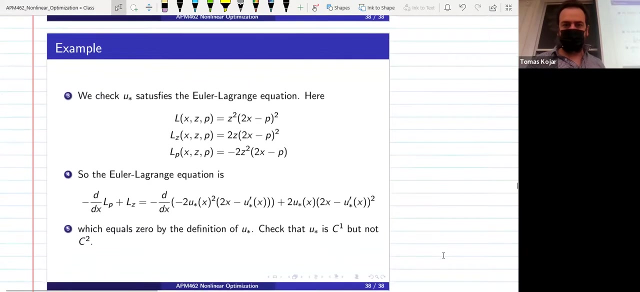 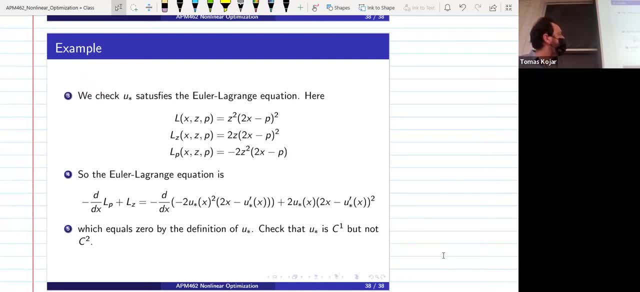 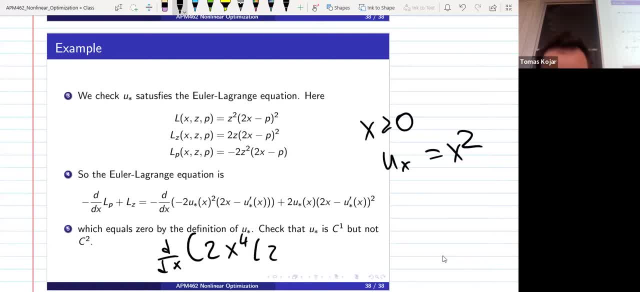 Okay, x to the 4, 2x minus 2x, So it's 0, right, Yeah, Okay, So this guy is dead. And then you have 2x squared. This is again dead. Yeah, so these are both dead. 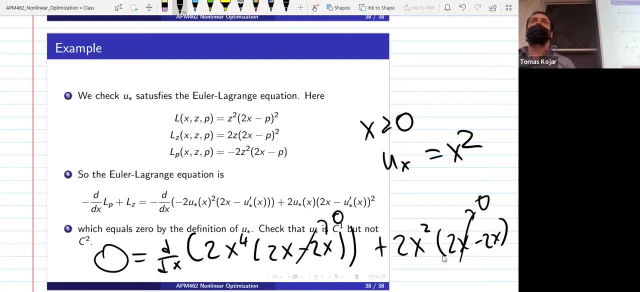 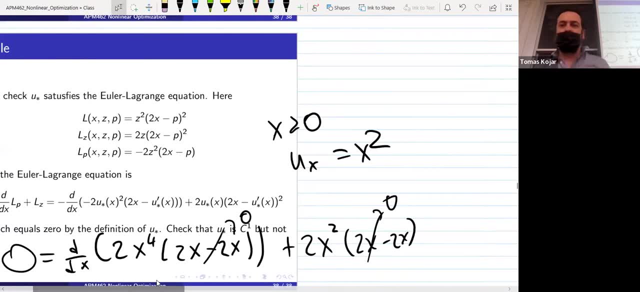 Okay, so it is a solution in a stupid way, And. but then the 0 function is also a solution. So for x negative, if you put u star equals 0, what do you get? So you get d dx 0 stuff and then plus 2 times 0 stuff, which is again 0. 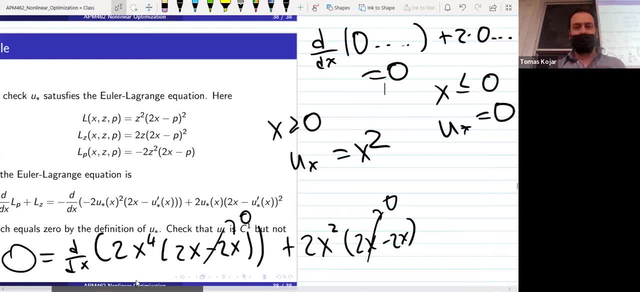 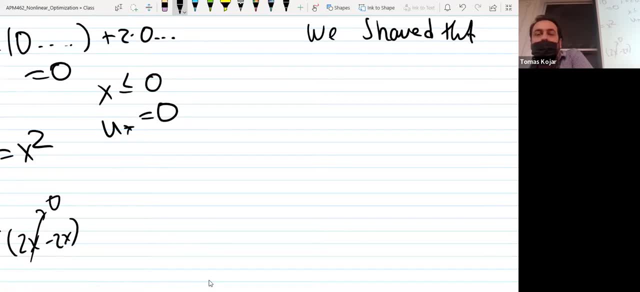 Okay, So now, why am I talking about this? So we just showed that u star is given by 0 and x squared. Okay, But then if you take two derivatives, what's the second derivative when x is uh? uh, no negative to what about uh here there? 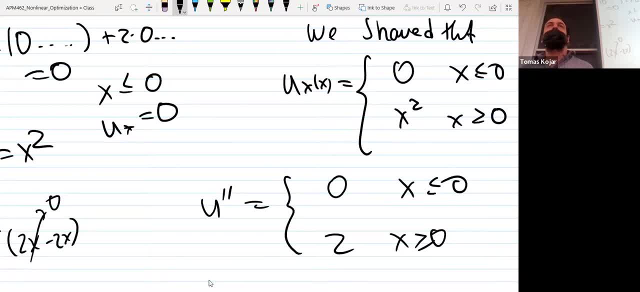 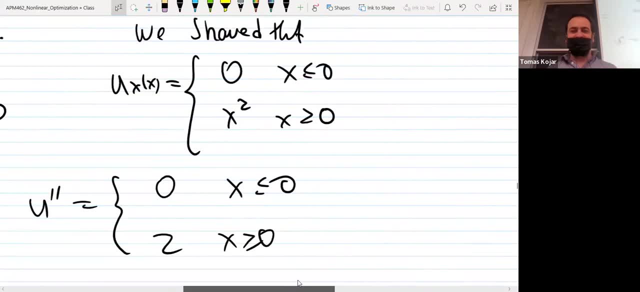 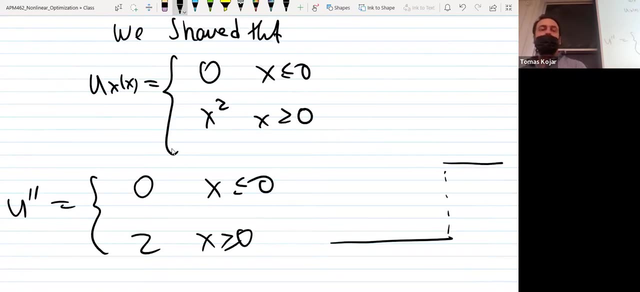 So is this continuous? Is it a continuous function? Yeah, What? No? no, I'm talking about u prime, u double prime. What So, what? Yeah, yeah, So so it's not continuous, so not continuous. 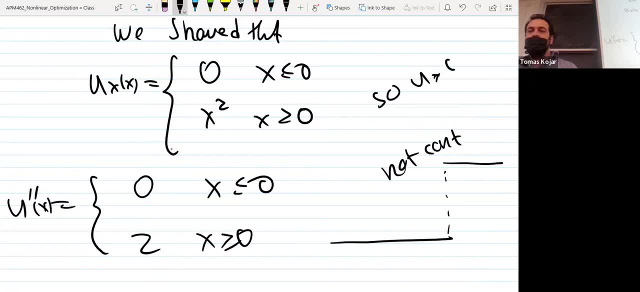 So uh, so u star, uh is not c two. Okay, so the the point is: um, the result would just prove: uh, there's a weaker version of it, Uh, but it requires more machinery. Anyways, 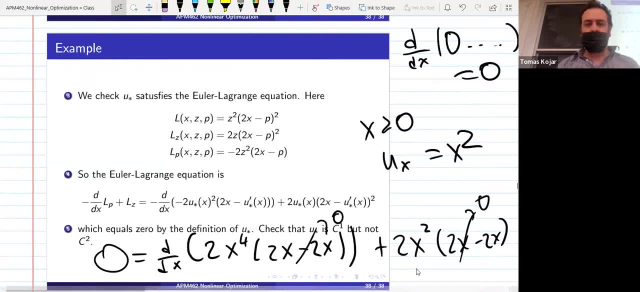 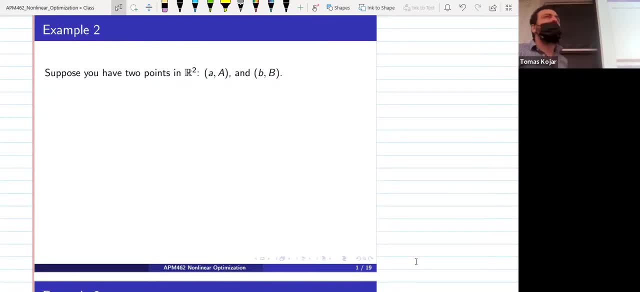 So give me, Please, give me. Uh, let's go. alright, no more examples. Um, So this goes under the name geodesics. I should have been this. Uh, being real, We probably have to learn this when you go and do jeerie. 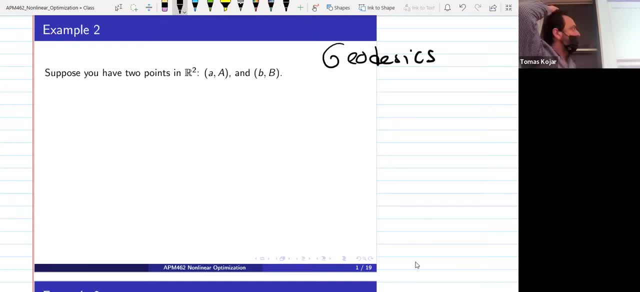 This will be your first. uh, we have a little bit of one class. we do rate of convergence, but i want to go into geodesics a little bit. so, anyways, this is in the book. um, okay, so in the plane it's easy. uh, the question of 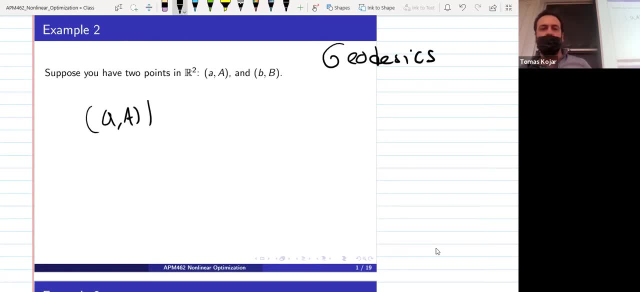 suppose i give you two points and i ask you, uh, what's the shortest path that connects them? is this the straight line? but what if you are? if you are in some other object, like a cylinder, and i give you two anti-anti-portal points, what do you think is the shortest path? 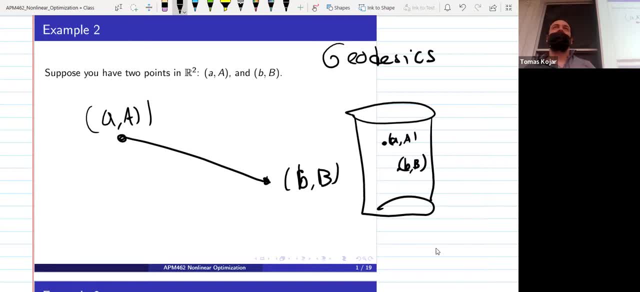 yeah, we can do with your hand or your pendant. oh, let's keep it down. i mean, i think you're, yes, you're getting close, but visually, like what do you think what's the closest path? so you, um, oh, i see, yeah, it is a little bit difficult, isn't it okay? yes, you're. 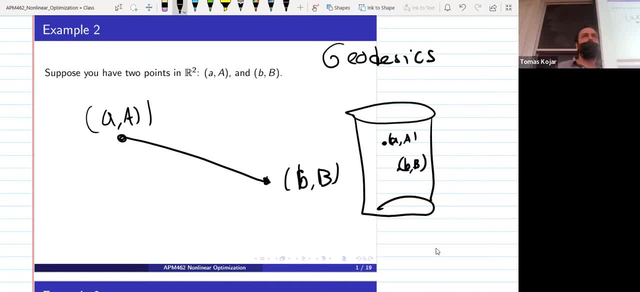 right, let me think: yeah, i said anti-portal, i said anti-portal, so it's easy, you just take um, you just take the, the equator, yeah, otherwise it's a little bit hard, you have to have some tilt it anyway. so this is a geodesic, okay, and uh, people want to find the curve, they want to. 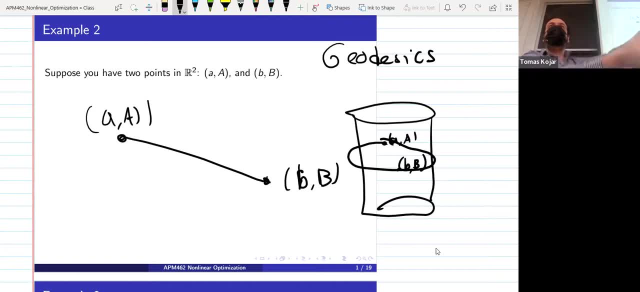 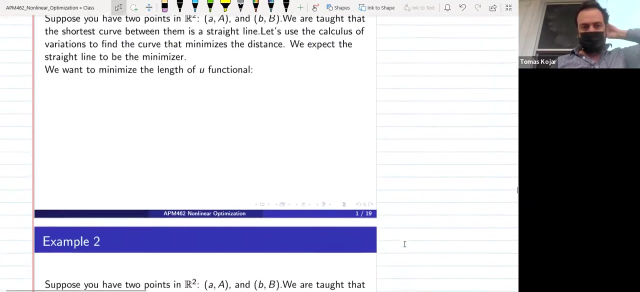 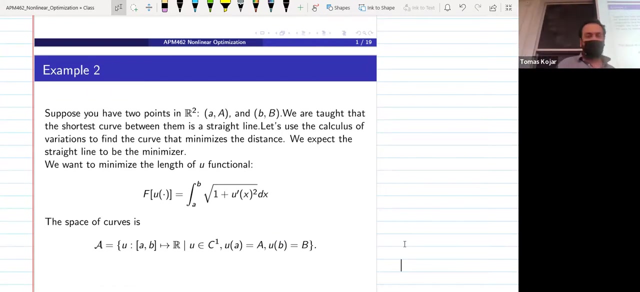 give them some constraints on your geometry. this is the functional. give me the path that minimizes the distance between them. okay, so yeah, good, so yeah. this is, uh, yeah, i want to explain to you, because many of you might not have taken geometry. so where did this come from? um, so a way to write this, as is one plus du dx. 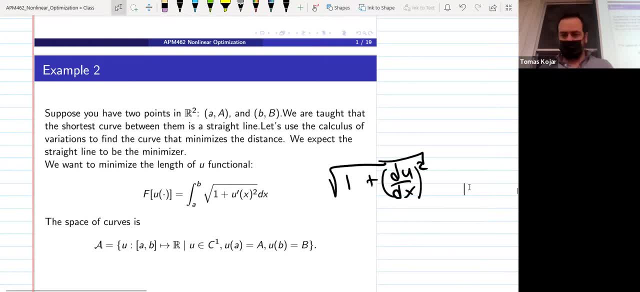 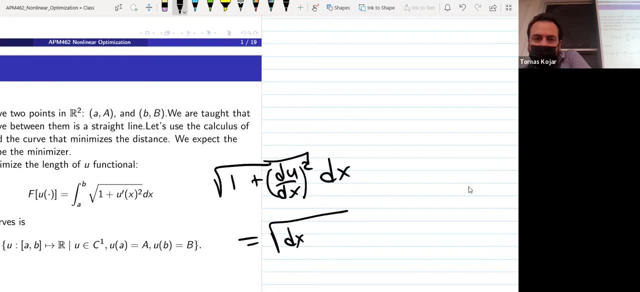 you factor out the dx and then you have: uh, dx over here, dx over here. they cancel out, so you get. so you get a square root of dx squared, du squared. does this remind you of anything? what's the if i give you two vectors in r2? 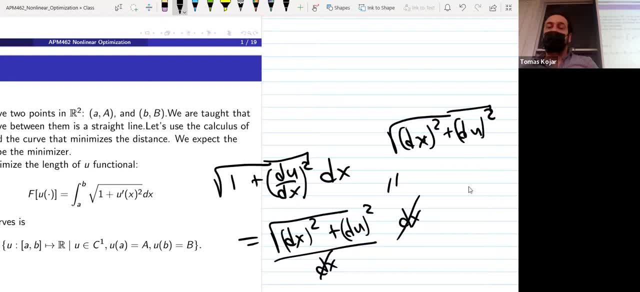 uh, yeah, what? yeah, yeah, so it's the euclidean distance. and uh, what was that? uh, if i give you two points distance of aaa and uh, bb is given by uh, what, yeah? good, all right. so all it says is: i want to minimize the uh euclidean distance and 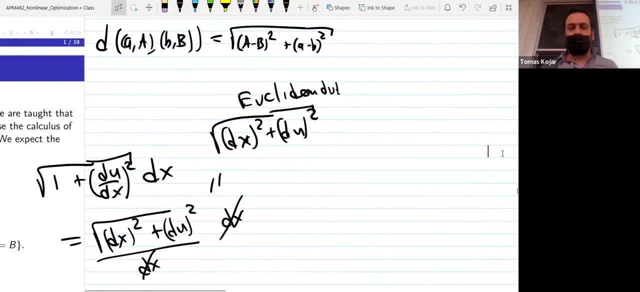 uh, i wanna in the future come back and do the more complicated stuff. so, instead of just euclidean, you add what is called curvature, and it shows up. here is uh, so uh. but we'll come back to it. so usually, Usually when you want to, when your geometry is different, 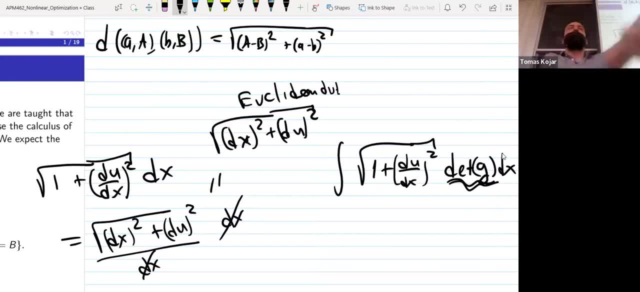 you pick up a factor over here because you do change your variables. So you change from like a flat guy to like the sphere or the cylinder And, if you remember, from change of variables you get determinant of Jacobian And that's basically: this is like determinant of Jacobian. 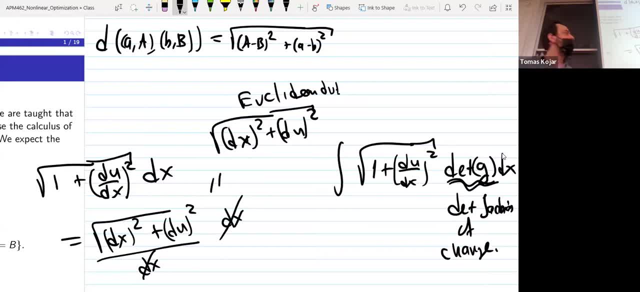 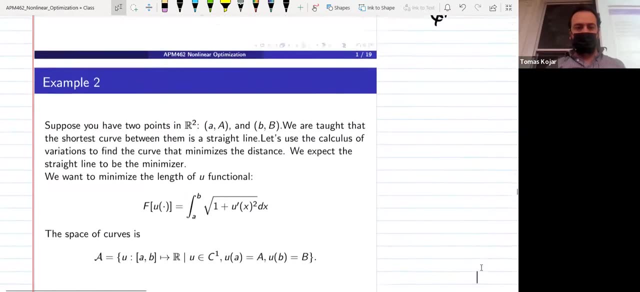 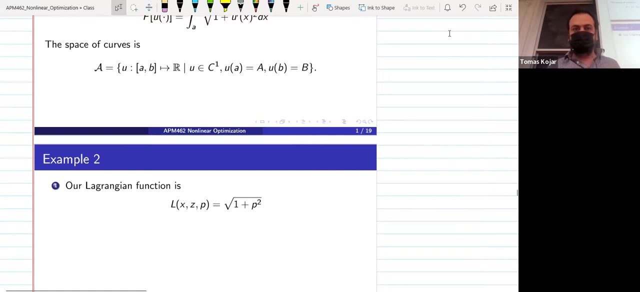 of the change of variables. It's really that simple. it's not very complicated. All right, I want to do the cylinder example next week, All right? Okay, I wish I asked you, but okay. So this is my functional and I want to minimize. 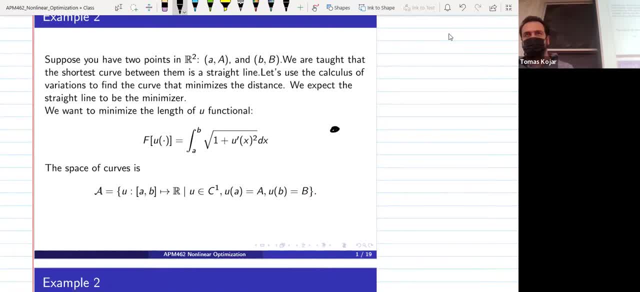 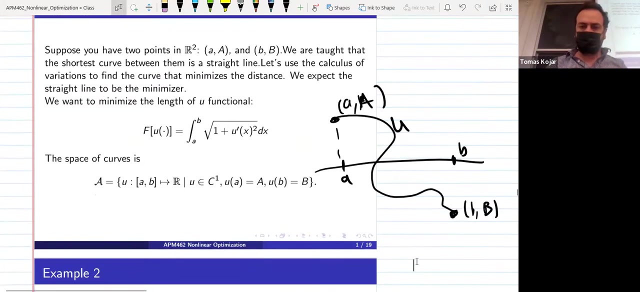 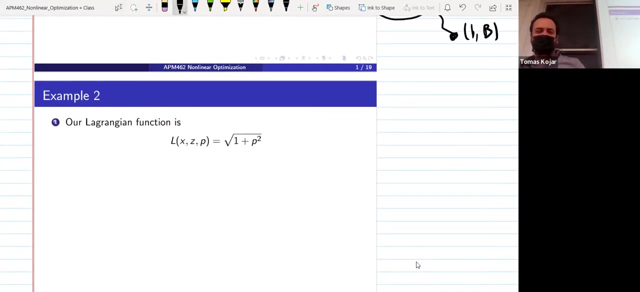 over all points, over all paths that take A and connect it to B. okay, And we will prove that it's just the line The Lagrangian is given by this. Let's do it together, all right, Bort. 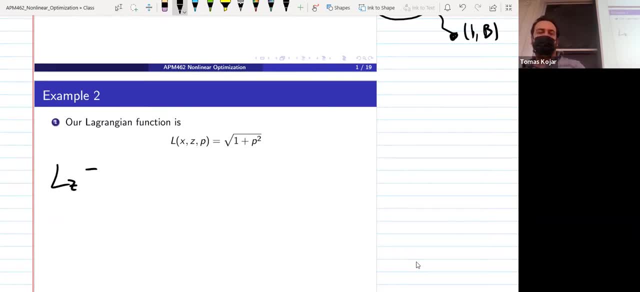 So what is that L of Z? Yeah, what is L of P? What do you think? Let's do a little bit simpler. first, What is the derivative of square root of X? Is that okay? So you just do chain rule. 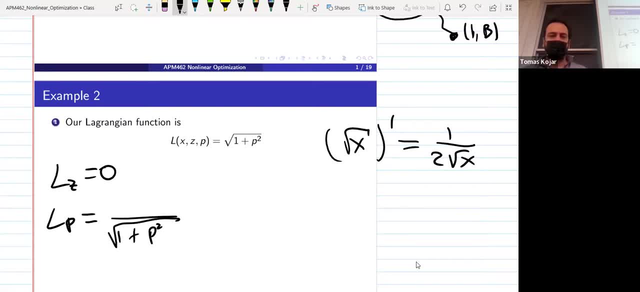 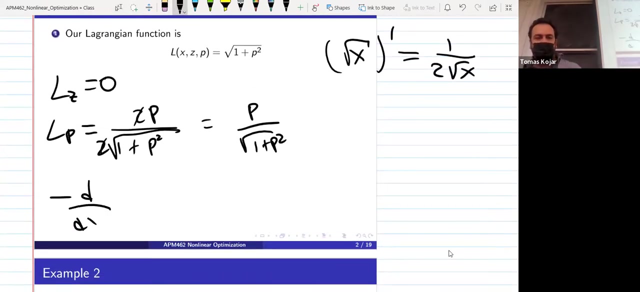 So you get your guy, And then you do chain rule, So you get two P. So yeah, All right, And let's go. So then you have minus D, D, X, L P for P equal to one, All right, So what? 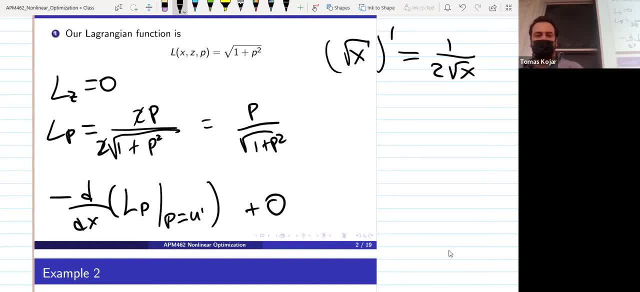 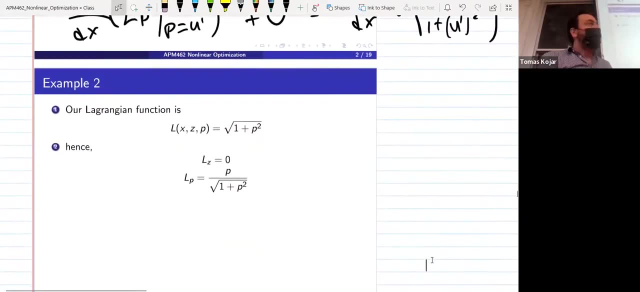 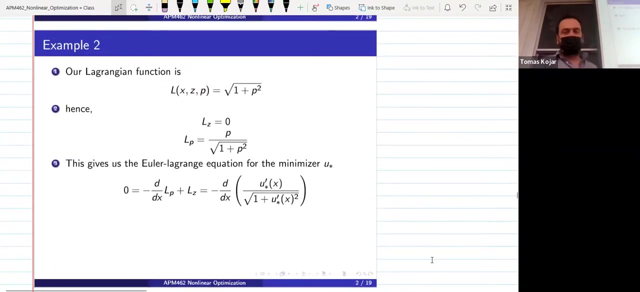 Yeah, U prime plus zero, right, Okay. So then you have minus D D X of U prime over one, plus U prime squared, All right. So, yeah, this is L P and this is your OD. it looks absolutely terrible, but we will try to solve it. 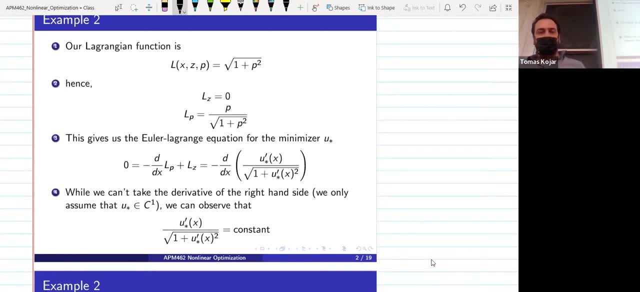 So one thing that, yeah, So here we're kind of lucky, LZ was dead. That's very nice. So that means that you have a derivative guy. And remember from first year it says that whenever you have F prime to be zero, 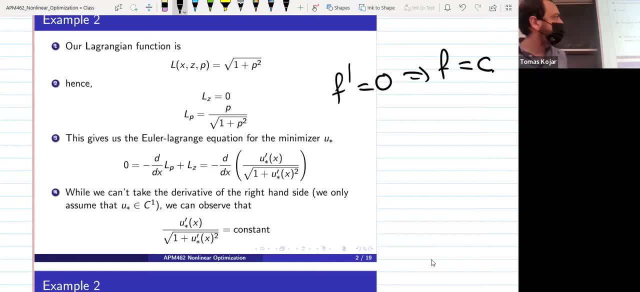 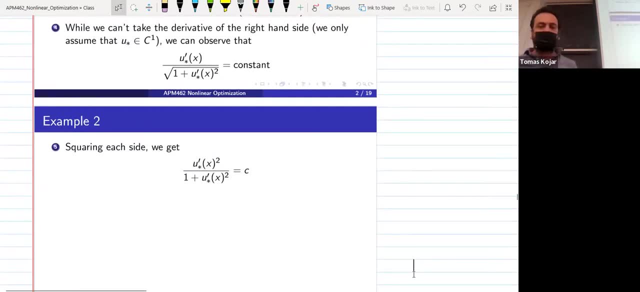 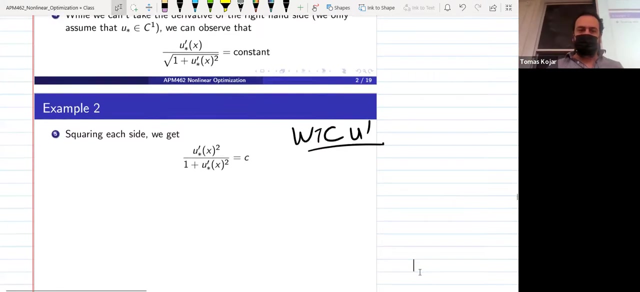 F needs to be constant. Yeah, So that's all we're saying here And now. I want to find U prime. I want to find. I keep writing W want to want to compute. Yes, I want to compute U prime. Any question? 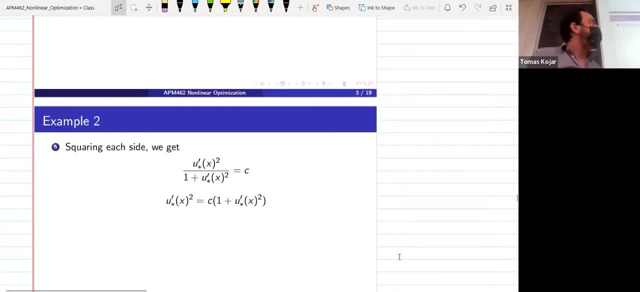 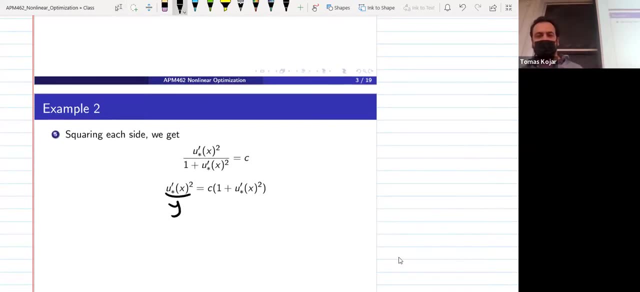 So then okay, So Yeah, I isolate. then I have one unknown. Okay, I can show you, but we can do it together. So call this guy Y. What do you think Y is? I don't want to keep looking on board. 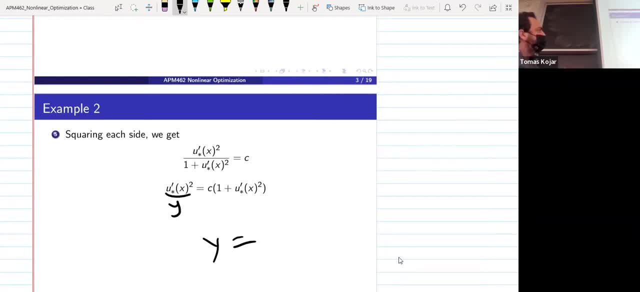 So Y is equal to yeah. What do you think? I mean, don't look, I can look as well- What do you think? What is Y? What's your guess? Yeah, What's your guess What? So, yeah, we have to assume first of all. 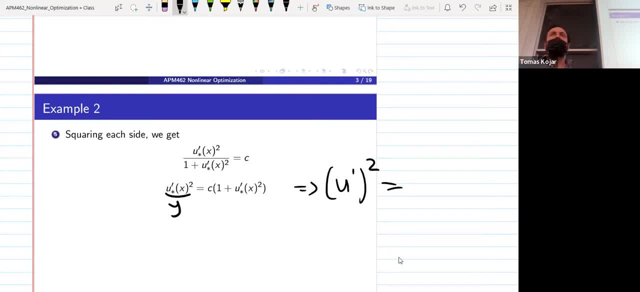 so what can we say about C just from here? Can we figure out some things about C, like the domain of C, Like Lafley, what do you think? Yeah, it has to be less than one and it has to be positive, right? 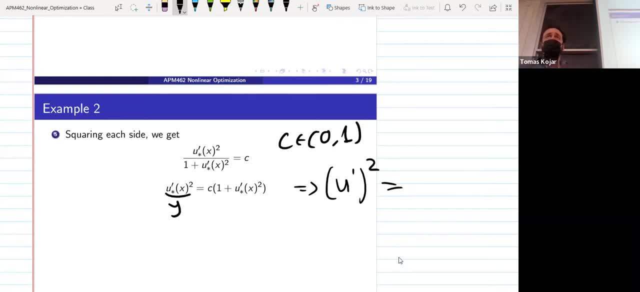 So it has to be strictly less than one. So then I'm allowed to bring this to the left and divide by one minus C. Is that okay? Is that okay? All right? And now you, yeah, you- do your square roots. 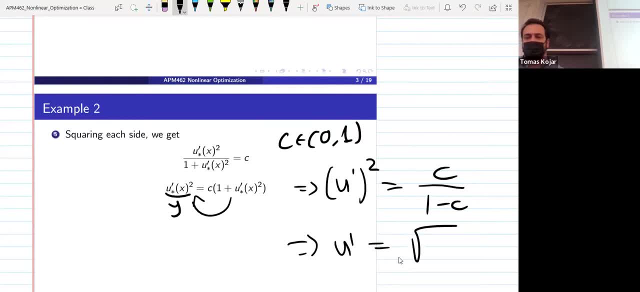 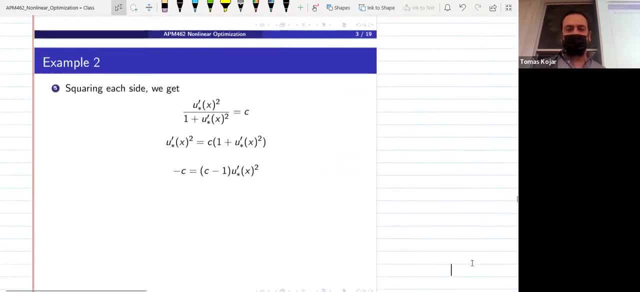 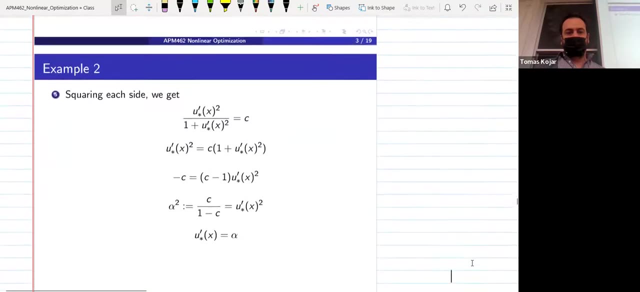 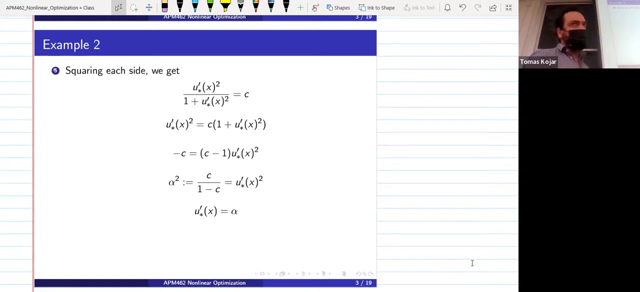 But this guy is positive, so it's fine. And anyways, from here I think it's clear, We just integrate. Yeah, So you have U prime equal to this C, square root of C, one minus C, and I just integrate. 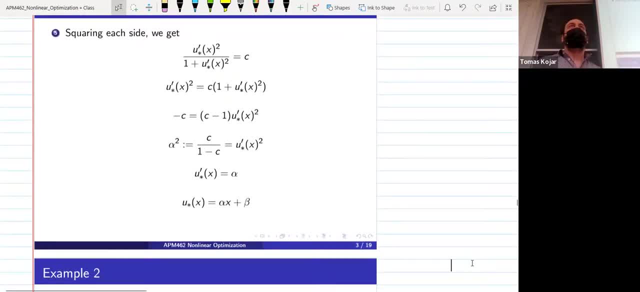 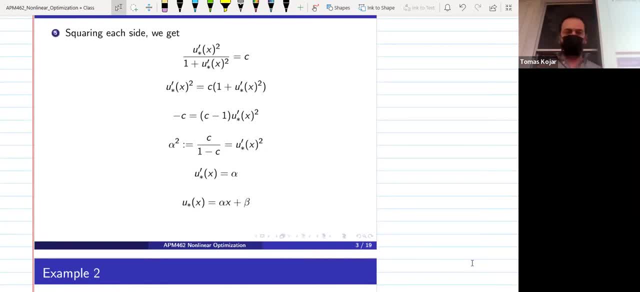 And that's exactly what we expect it to get the line. So let me find the alpha and the beta. So we have that U of A is A and U of B is B. So we have that U of A is A and U of B is B. 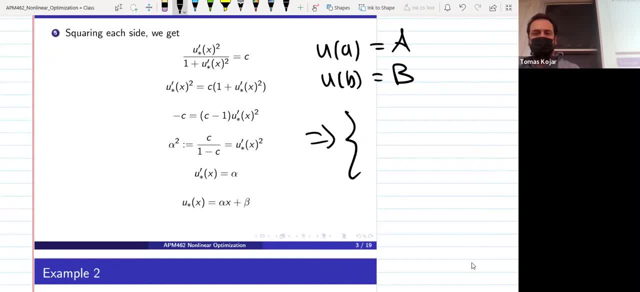 So I have the following system: Too many alphas, So this is alpha of A. I hate this. No, What's another good notation? What's another good notation? it'd be like px plus q, i don't know. okay, well, who cares? so this is p of a plus q is a and. 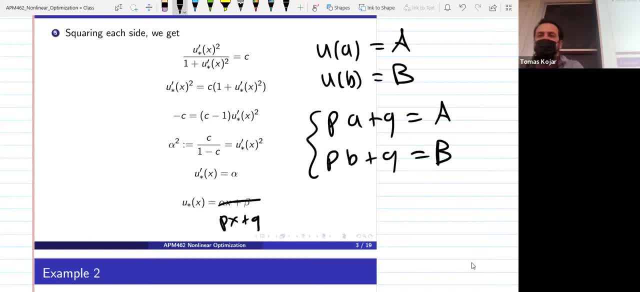 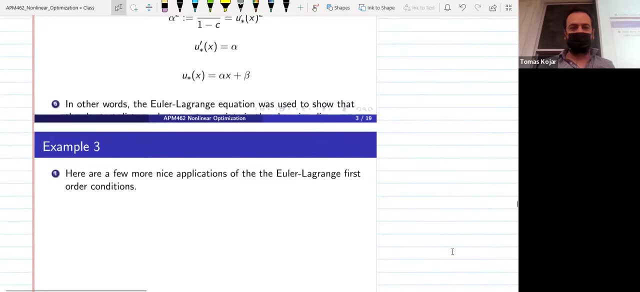 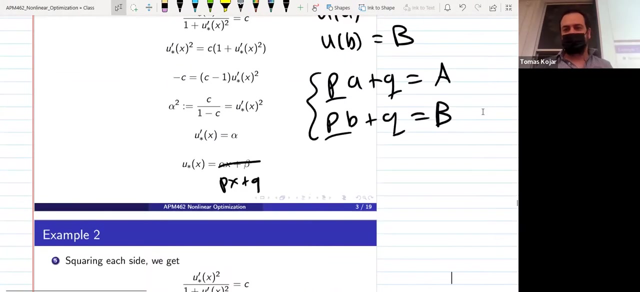 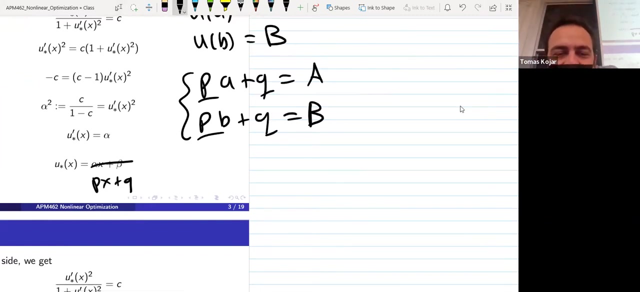 pb plus q is b? um. two equations, two, two unknowns, two equations, and uh, do i want to solve it? okay, oh, i missed my slide. okay, we'll do it together, uh, so okay, let's go. is there an easy way to do this? maybe, uh, subtract them right, so you have p of a minus b. uh is equal to a minus b. 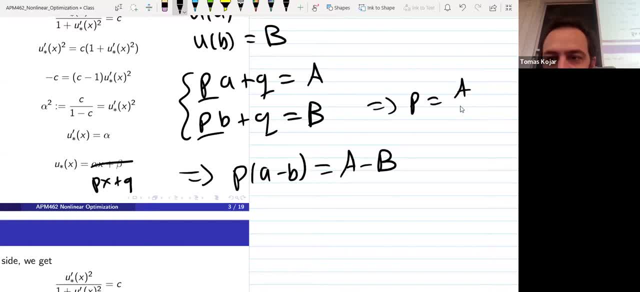 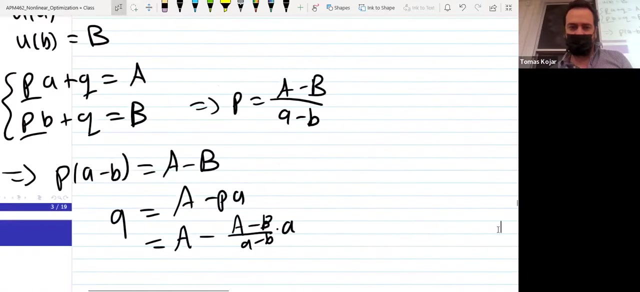 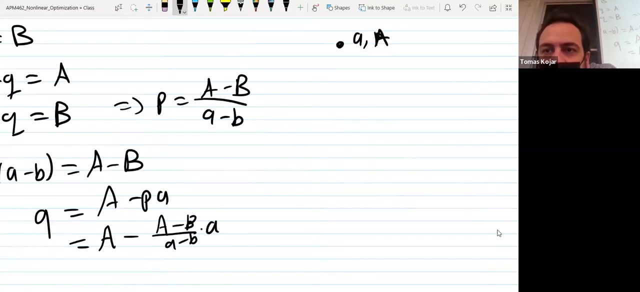 so i get uh p right, which is the slope from um high school and then um and then q um. i know it's equal to pa. no, yeah, a minus pa. so it's terrible, it looks terrible, it is what it is. so then will this work? so it says that the guy who connects a, b, uh, a, a to uh. 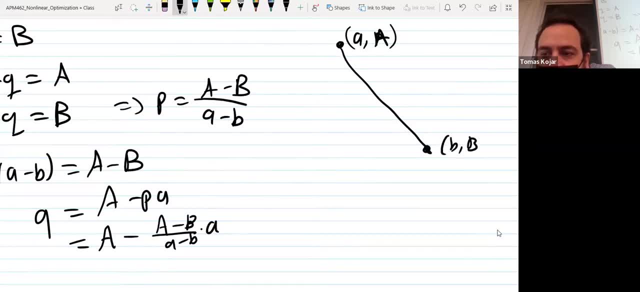 bb is given by the line y equal a minus b, abx, and this is the intercept. do i have to write it? i mean, that's the intercept, okay, does this give? Does this line connect the two? So let's, I mean, I know that this is the right slope. 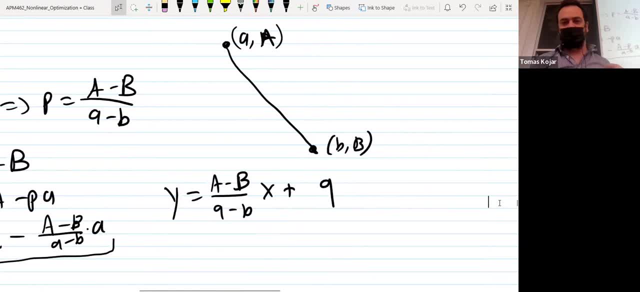 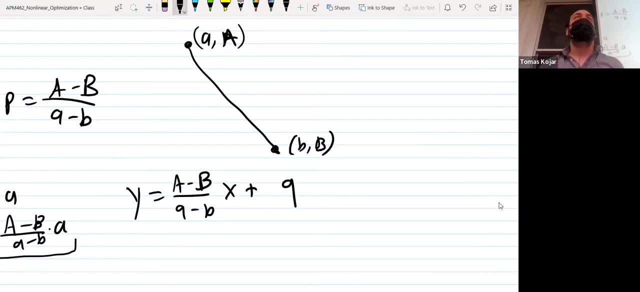 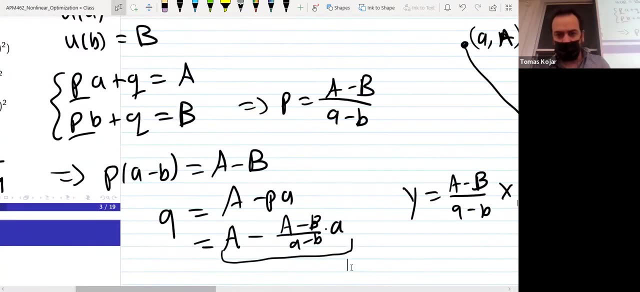 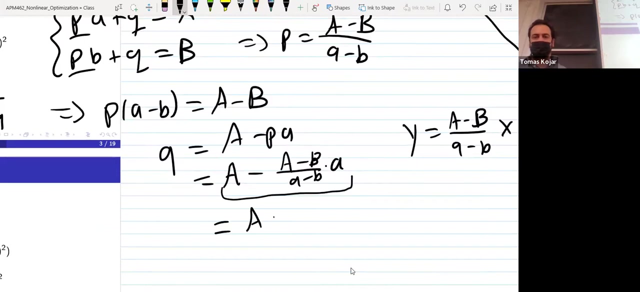 but I don't remember the intercept. Sorry, what Does it have? a nice formula, Don't worry, don't rush. So you said it's big A, Sorry, what Times? small b, No, Well, I think I know what you're saying. 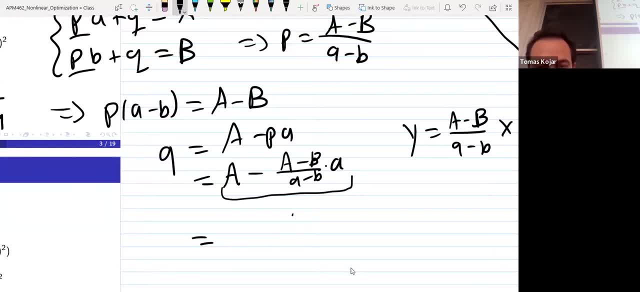 Yeah, there's a cancellation, So let me do it. So you have A A minus A, B minus A, A, A plus B, A over A minus B, And these two guys cancel out. Oh, I see, I see. 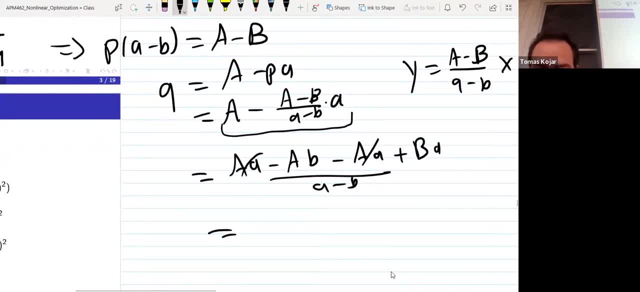 All right, I'm too, I should have done it All right. So this is B minus A and this is no, no, no, So I mean, it doesn't seem. yeah, I mean all right. 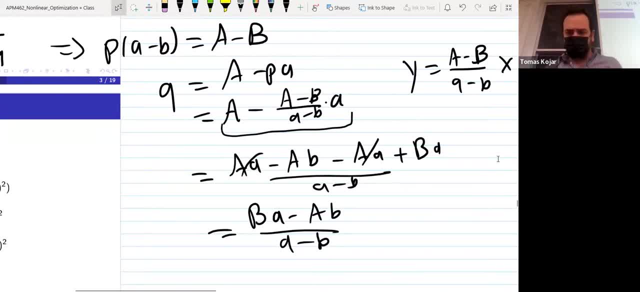 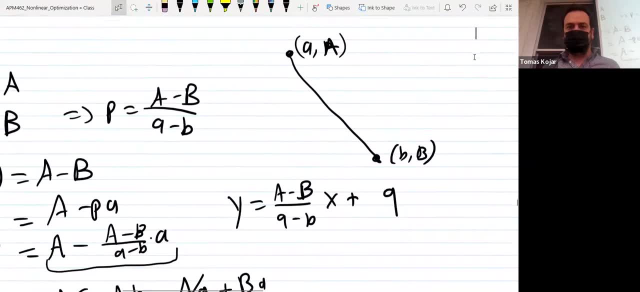 Yeah, yeah, okay, Anyways. so let's check that. this is indeed I want to check. let's check that this connects the two points. So what you have to do is you plug in X, equal little a. you're supposed to get big A. 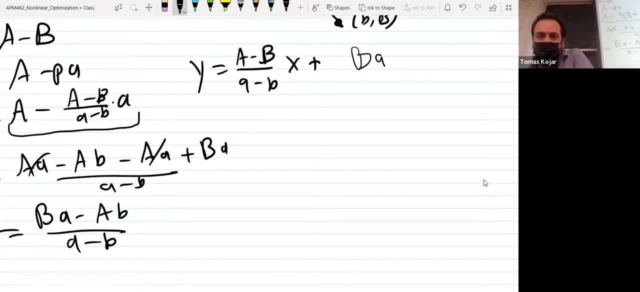 So let's go, let's do it. So if you plug in X, little a, which looks terrible, Oh, I liked it in the other form, I was right. No, you made it worse. It was way better, because now the cancellation is yes. 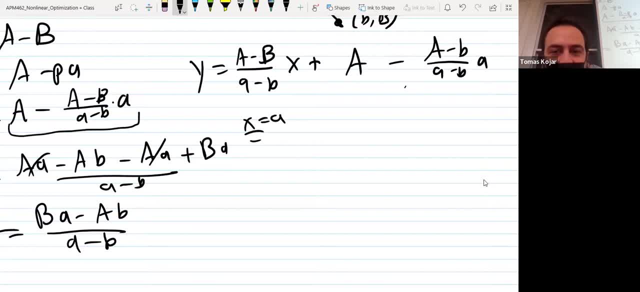 I mean, it's only easy in one case. In the other one your formula is actually better. So you have A, B, A, B A plus A, minus A, B, A, B A, and they cancel out. 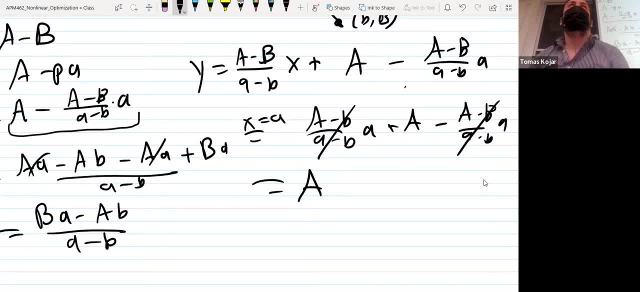 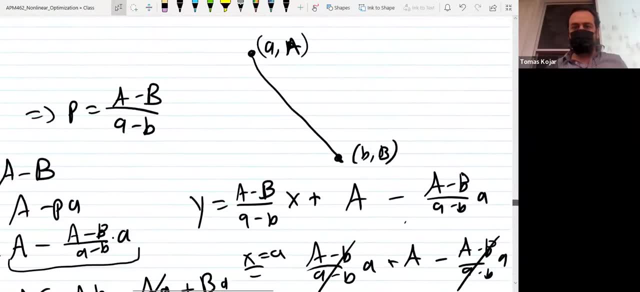 So you get A as expected, And then I don't want to do the other one. You could do it, But anyway. so this guy will connect the. it's just the line connecting the two points. All right, Now you get me curious. 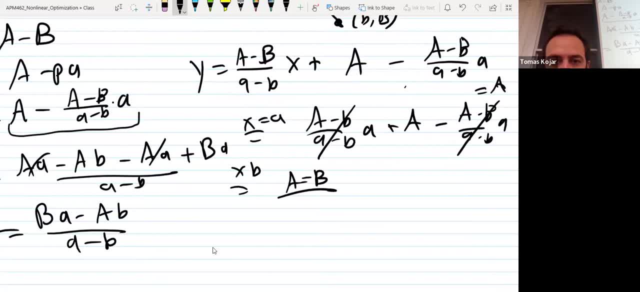 What if I put X equal B? So I got A B, A, B plus A, and this guy is the same factor. Now I see there's a cancellation. So you have A minus B, A minus B, but then you have B minus B. 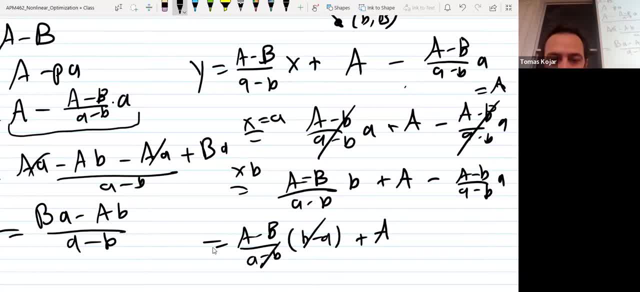 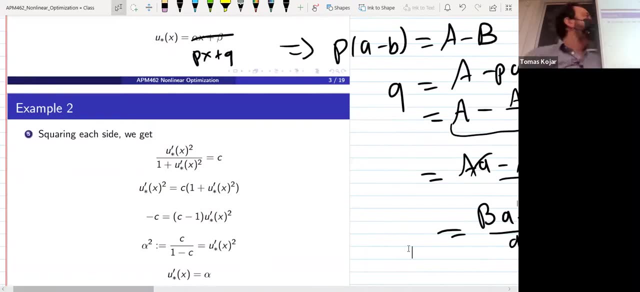 A minus A plus A, right, So you get B plus A minus A. So you get B. Okay, All right. good, Who cares? I don't really care about this, I don't know why. Too addicted, Okay, well, any questions? 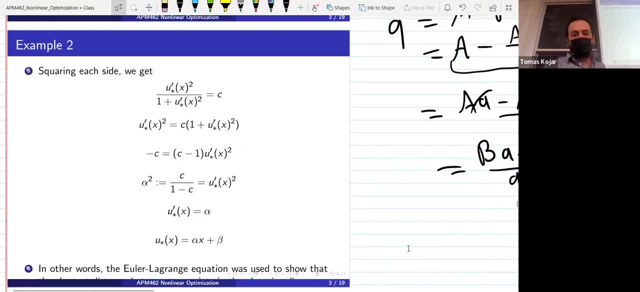 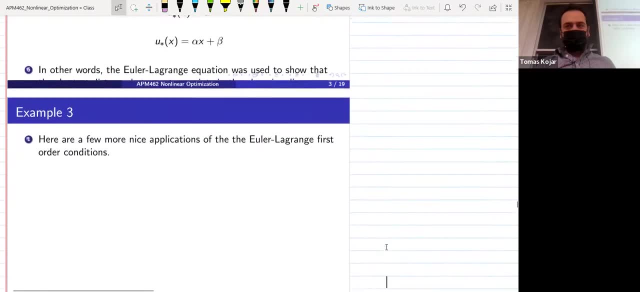 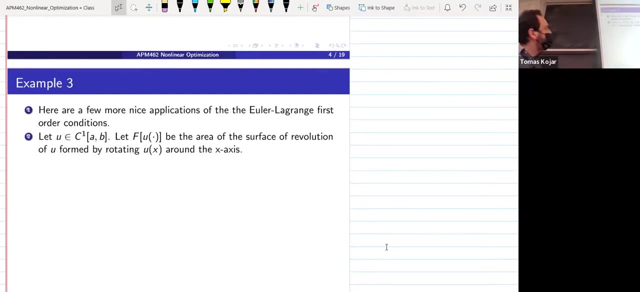 Other one works too. Yes, thank you, Daniel. Other crazy people like me exist. All right, Let's do more examples. Oh yeah, we're gonna do the cylinder now. I like that. So yeah, the surface of revolution of U. 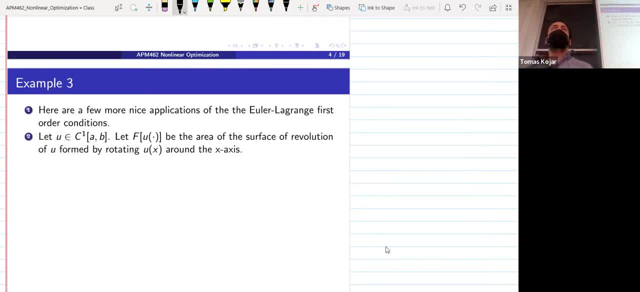 formed around the X-axis. Can anyone tell me how to draw this? How do you think it looks like? So here's the X-axis. Yep, very good, Yes, thank you. Do, do, do, do, do do. 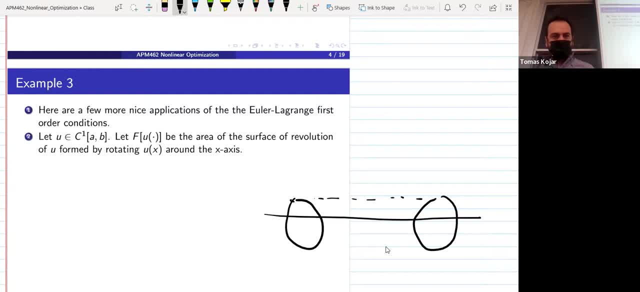 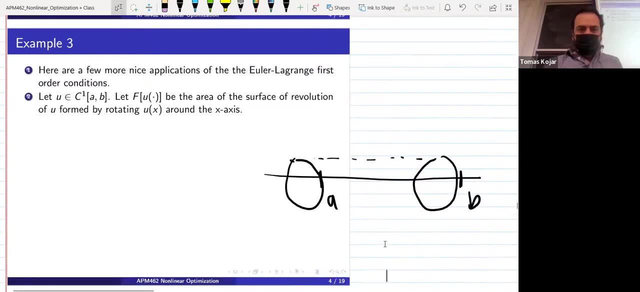 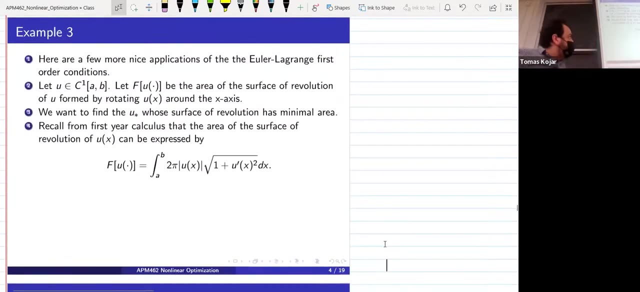 That's why it looks like this guy. Let me try that again About this guy. Like this guy From A to B. Oh yeah, Right, So you see my. I have my Euclidean distance and this guy over here is my change of variables. 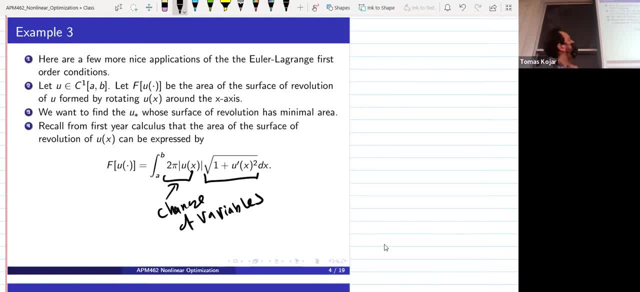 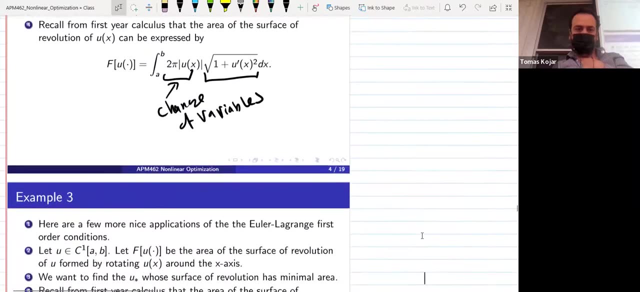 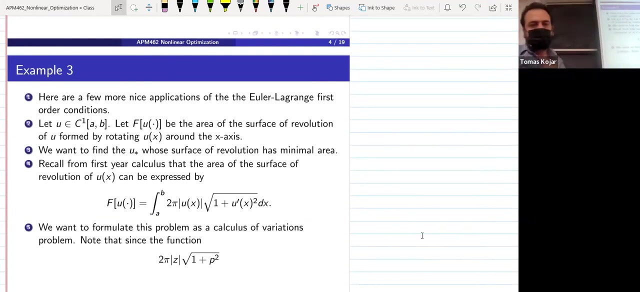 I want to see how Eric E should go. Oh, that should be okay. Who is my ravago? So let's see a little bit how I got this. so maybe too much. It's okay, it's a little bit, I'll do it next thing. 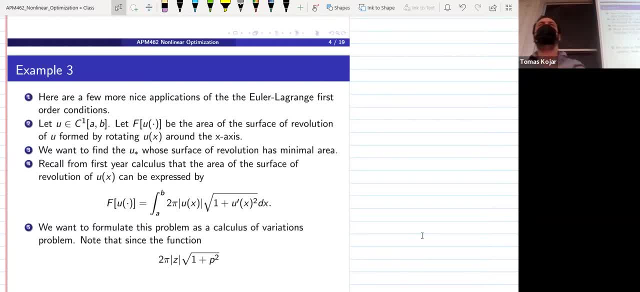 So so this is second year calculus material, And if I give you some graph, then yeah, you, you get this base. No, Is that okay? Yeah, so this is the surface of revolution. The other one was: So when you have access this constant. 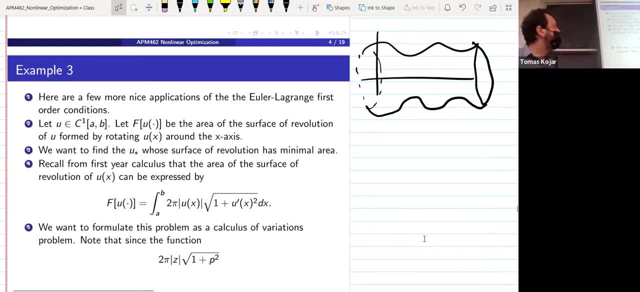 Yeah, we get the base And apparently I don't remember how you get this. I can probably do it by hand. I don't want to. So the surface area of this whole thing. Can we eyeball it why this is true? 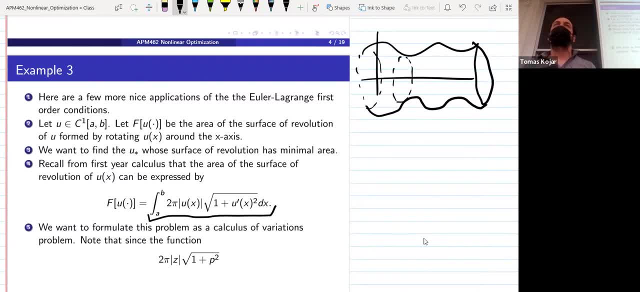 So this is Yeah, okay, go ahead, Right. So if you have x, that's right. if you have x was constant. I guess I'm trying to remember how do we get this. this is the Jacobian right. The slope- Yeah, this is the Jacobian right. the change of variables. 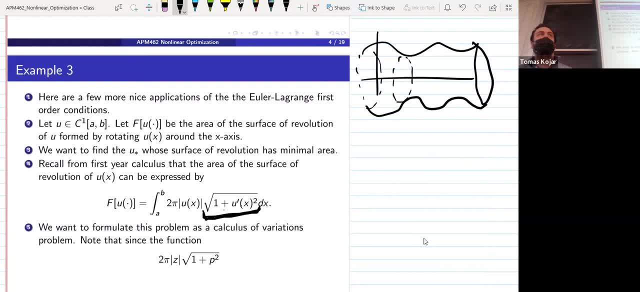 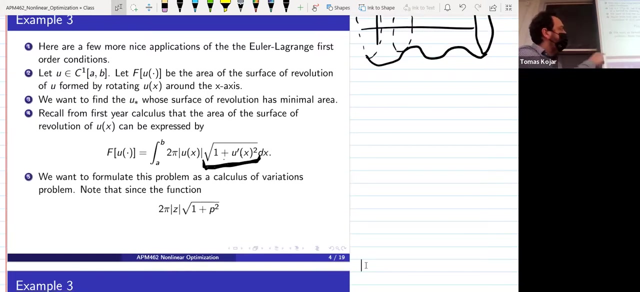 Right, So it should be something like: okay, I don't know, whatever, We'll do this again. Yes, okay, I have to stop. So, yeah, the Jacobian is given by- sorry, the Lagrangian is given by this function. 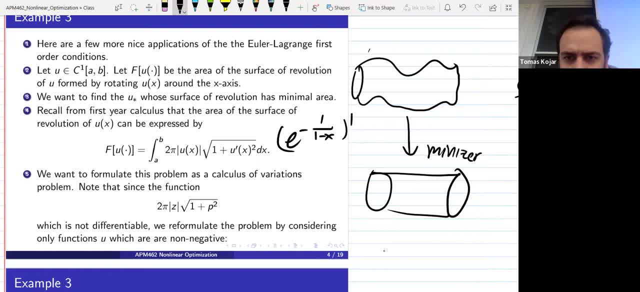 And then the derivative of that. You just get polynomials of it. Oh, that's interesting. Oh, I think it should be one minus x squared. Yeah, that's one minus x squared. Yeah, No Right, I was wondering if the square was inside or outside. 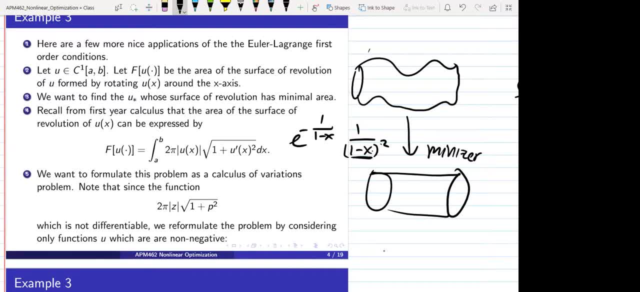 It's outside, because you do chain rule And the minuses cancel out. I'm not sure. I mean, there's probably another minus somewhere, Something like this: Yeah, Is this big? This goes to zero, doesn't it? But I think you're right. 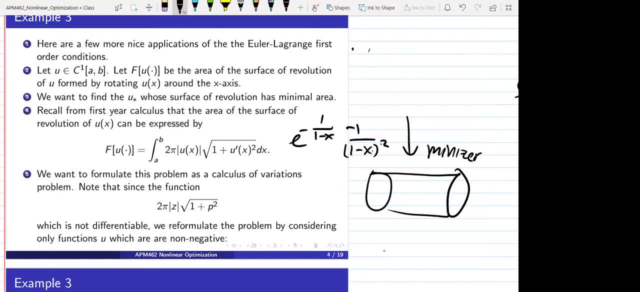 When you make this up, When you make this like sharp turn- I'm guessing someone over here- It should be like really big Right, Something should happen. Yeah, Can you play with it, Actually, if you're interested. I mean, it would be nice to see exactly. 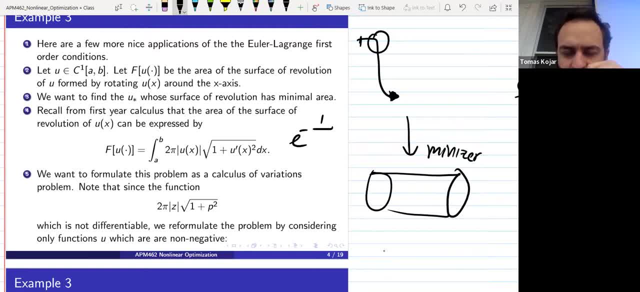 So this guy? what I'm writing is: So I want a B minus X, A minus B, A minus X, Sorry. So this guy is a bond function At a, B, Right And And then At zero You want it to be. 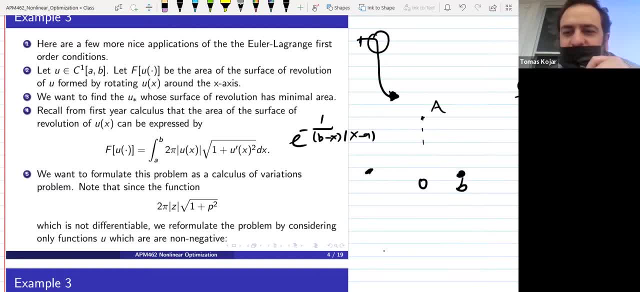 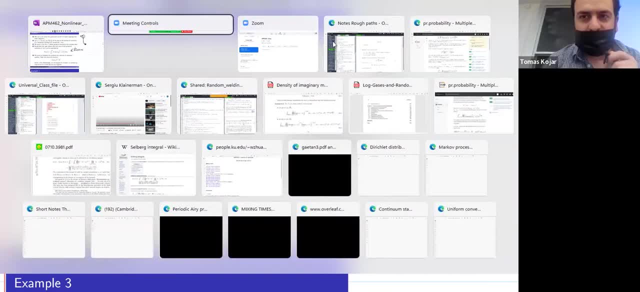 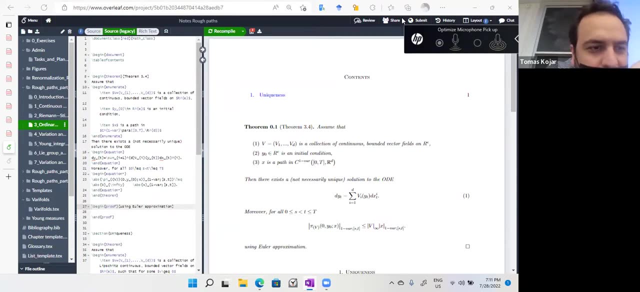 I guess a or whatever. Can you play with it If you're interested. I'll try Any questions. Oh, Daniel, Daniel, use your mic. I mean I can't read the. So one one minus X, Which way you go to one? 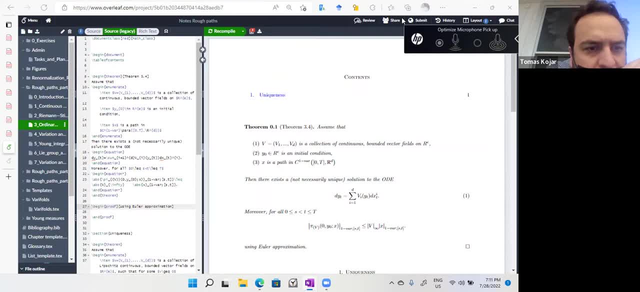 From one side, you go to minus infinity, From the other, it's infinity. No, no, no. We take X and zero one, Right. So And you come. Yeah, You come from the, From the left, Daniel. 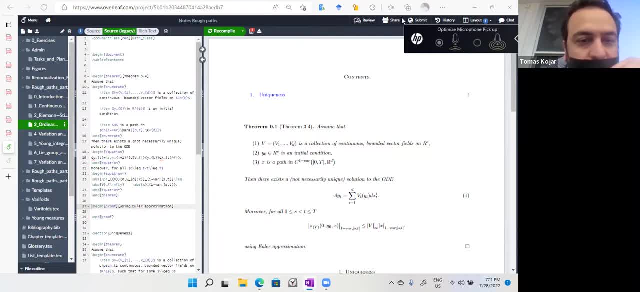 Yes, I don't know Where's Daniel. Daniel Right, That Yeah, We're not. Yes, And there's a second order. So But I don't, I don't, I don't really see it. 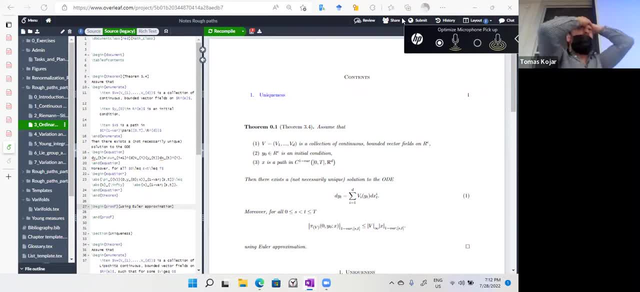 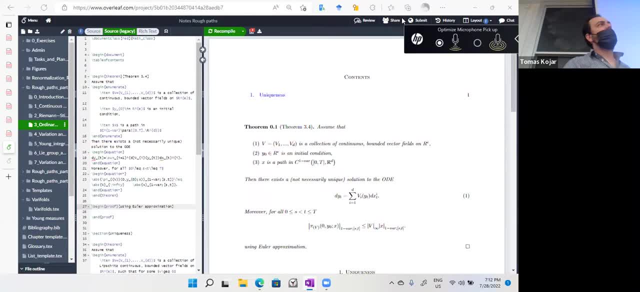 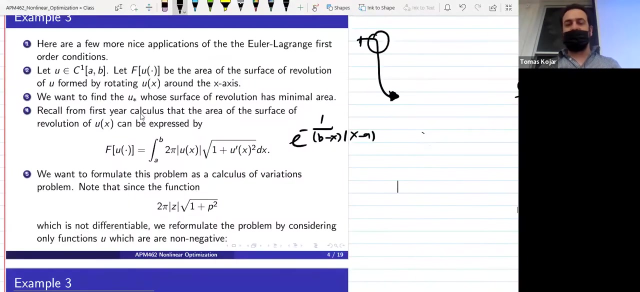 yeah, you need like convexity, so you have to look at the second variation, things and stuff. huh yeah, no, we're not going to do a second. i think it's deductible. it's like the action, remember he mentioned it. i mean, now you're. now you're asking. oh, i see what you're asking you're talking about. 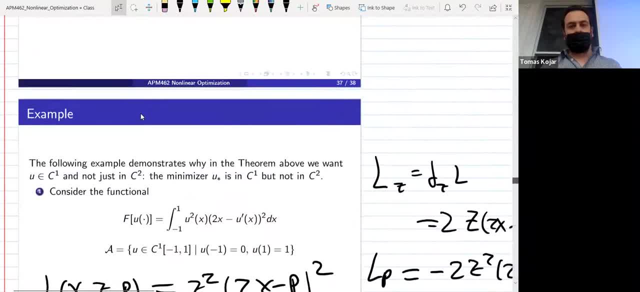 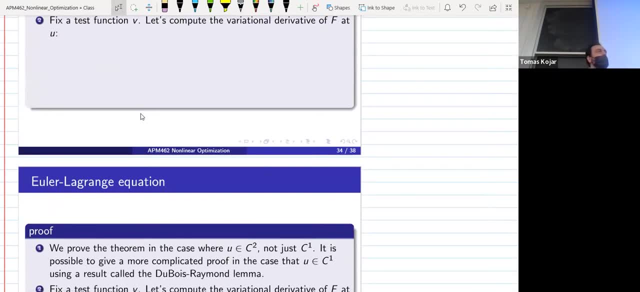 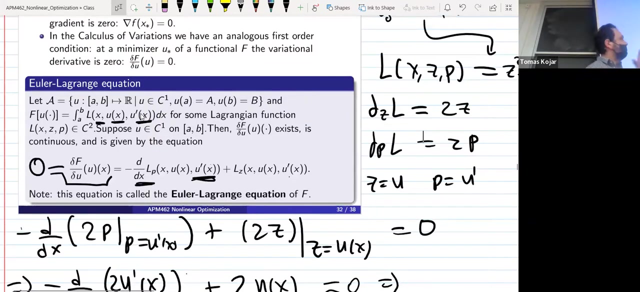 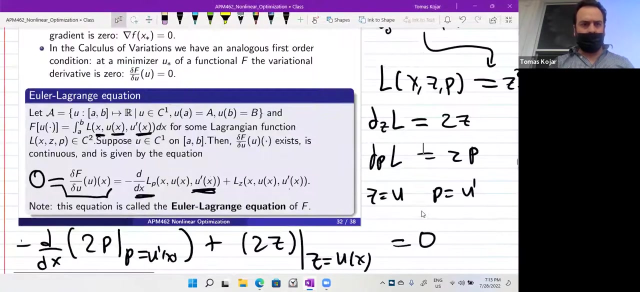 no, i mean, the least action principle is what i just proved, that the minimizer is given by this. uh, holy lagrange. so you have a. what does list action means? it means you have a conservation right. so this is the. so this is the like. uh, let's go back to that. 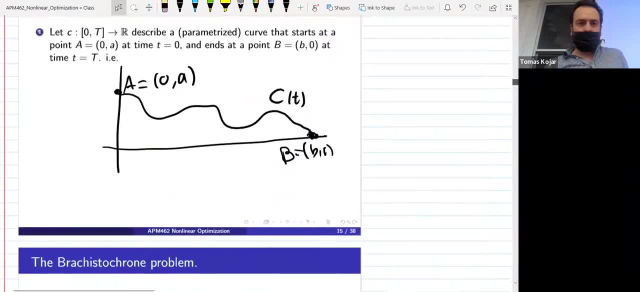 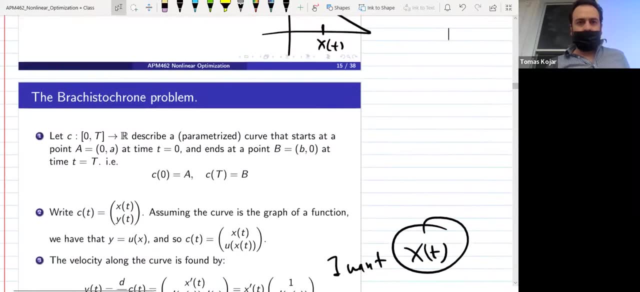 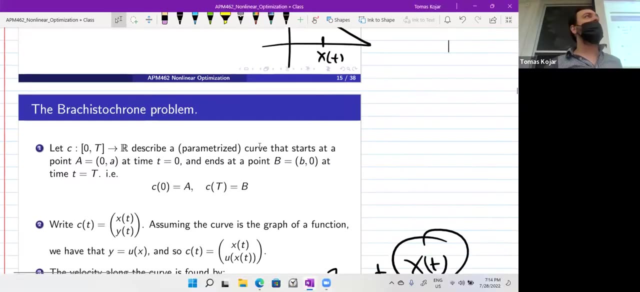 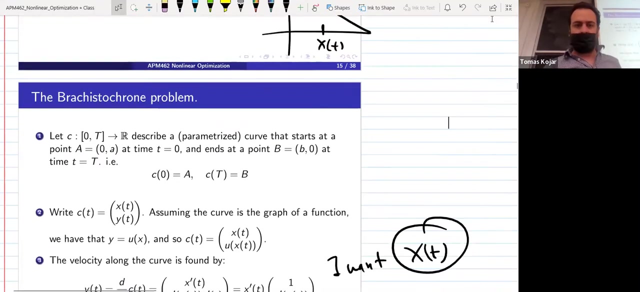 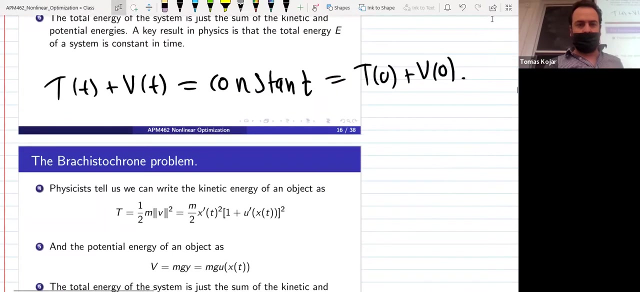 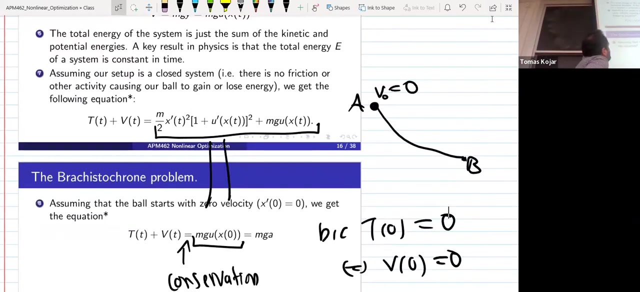 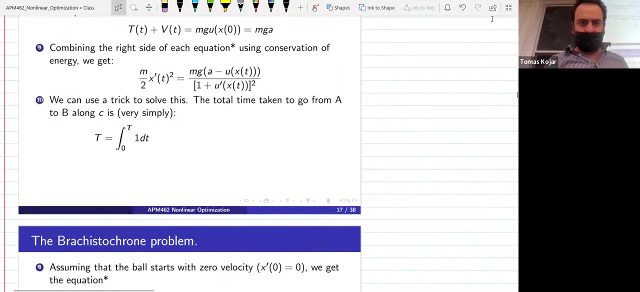 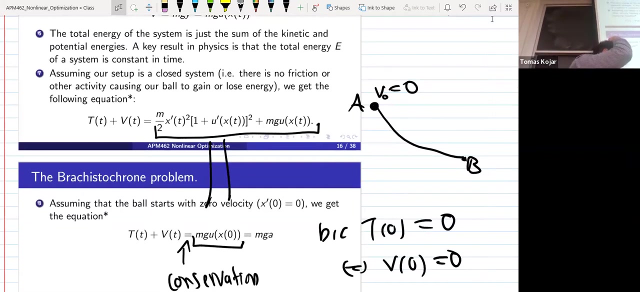 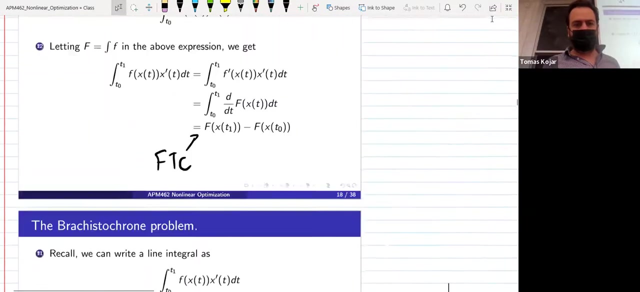 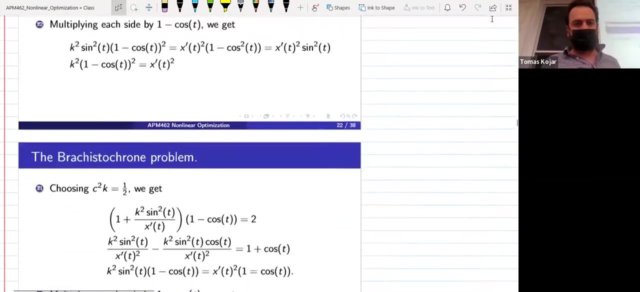 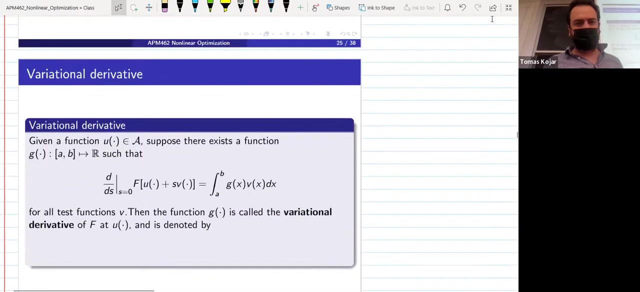 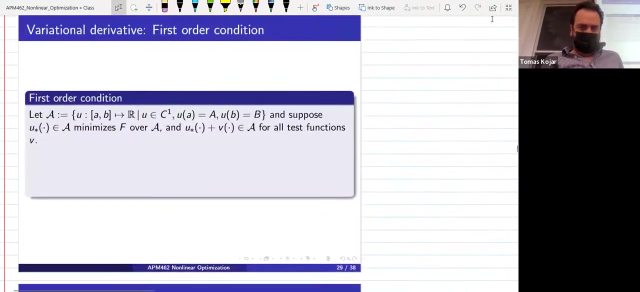 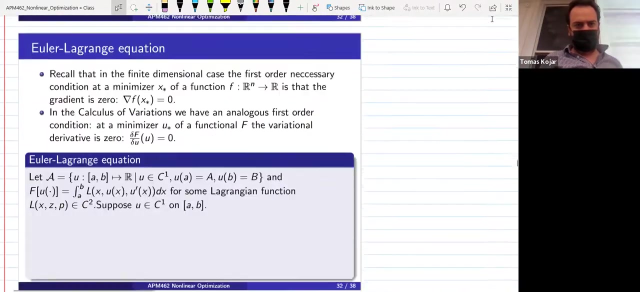 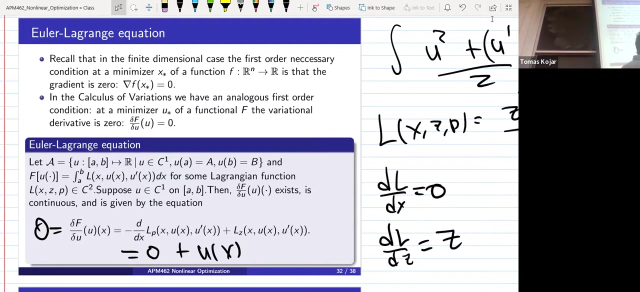 uh, there was a nice yeah, the brussels, yeah, like here, we had to use like a no, it's fine. it's fine, um, and i think this was a lagrangian right. so let me, let's go a little bit- um, um, so, so well. so at the back you have a Hamiltonian right and 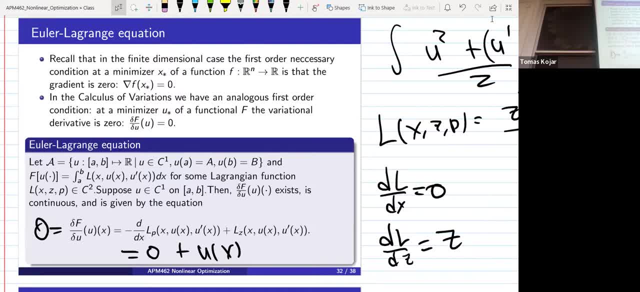 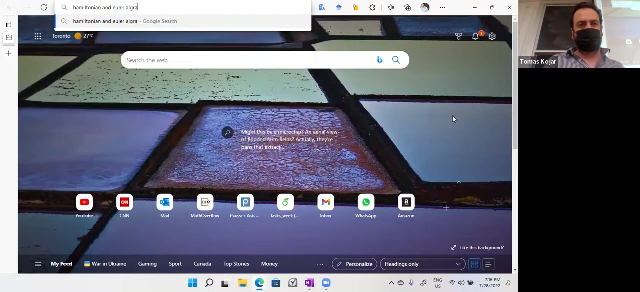 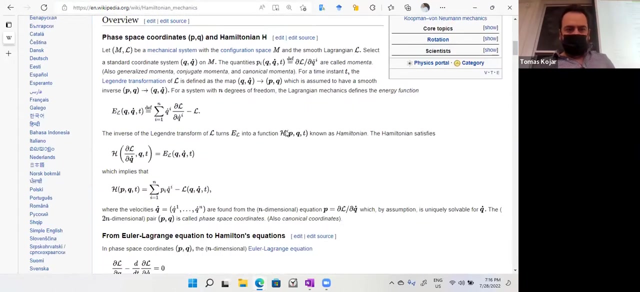 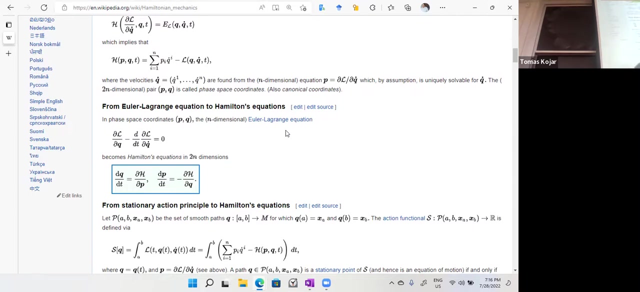 this equation implies conservation of that Hamiltonian. okay, yeah, so if you have, um, so yeah, um, um, um, yeah, um, uh, IHHHHHHHHH, IDt, uh, but anyway, so um, I think it's like let's just go around the people, People like a Jewish country, I don't know. 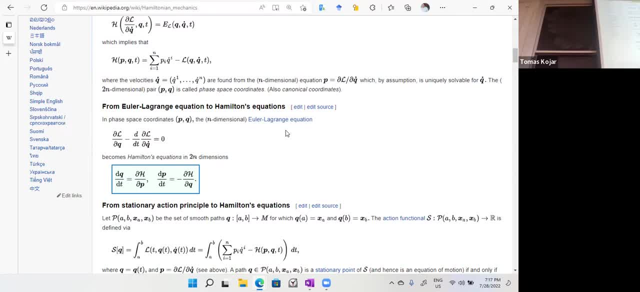 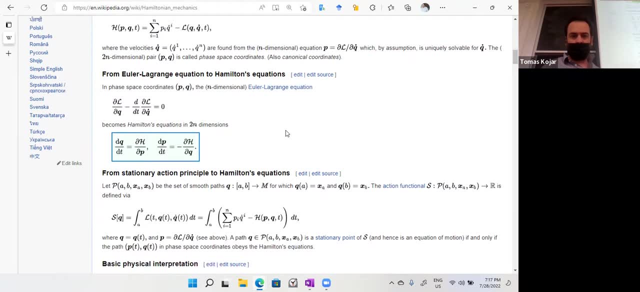 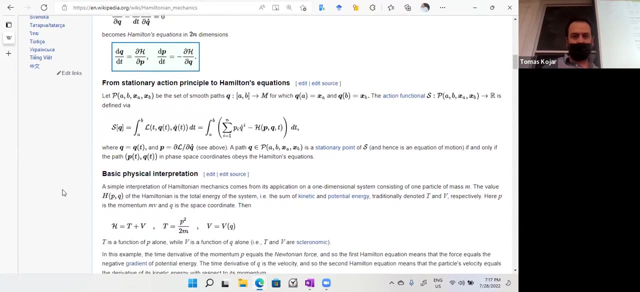 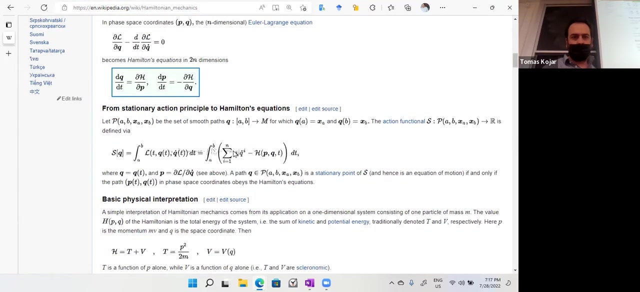 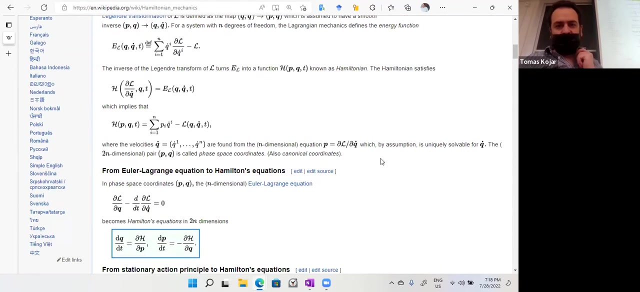 Do you remember? I don't want to. I think that's a good point, But I think that's how I would address that. That's a good point. I think that's a good point, But there was some conservation right. 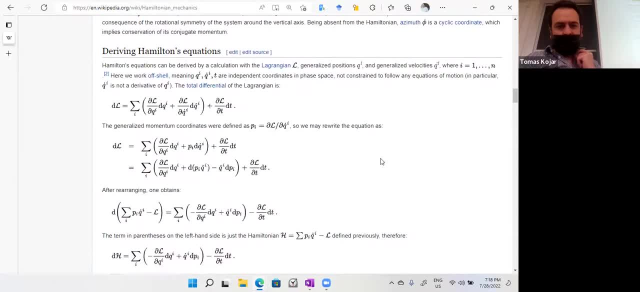 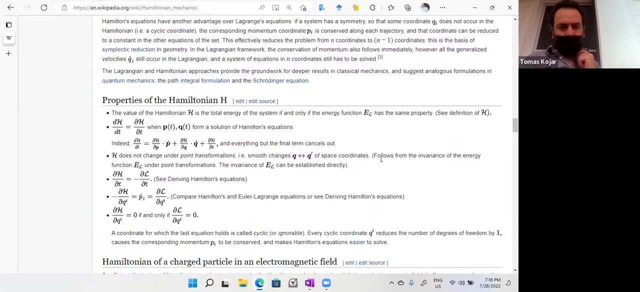 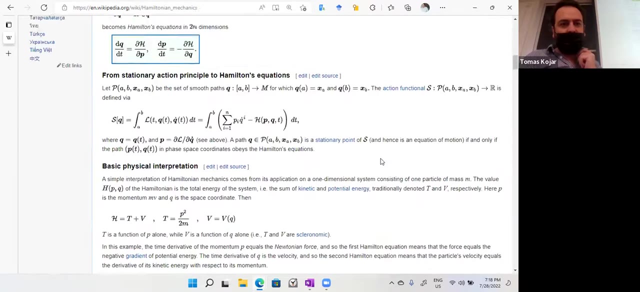 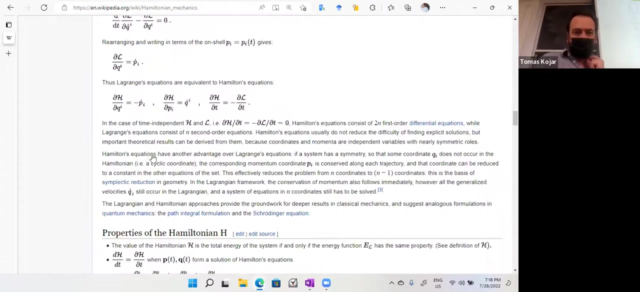 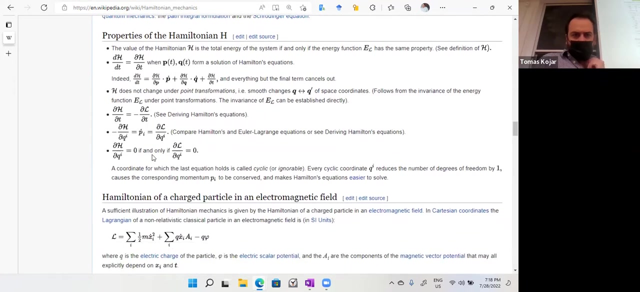 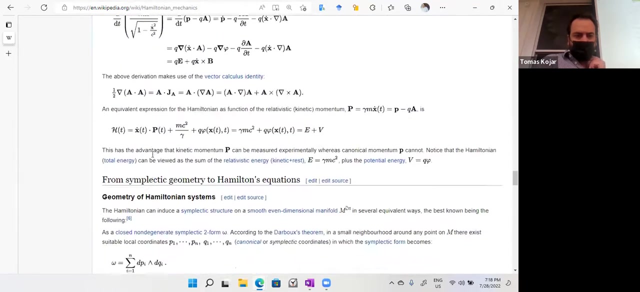 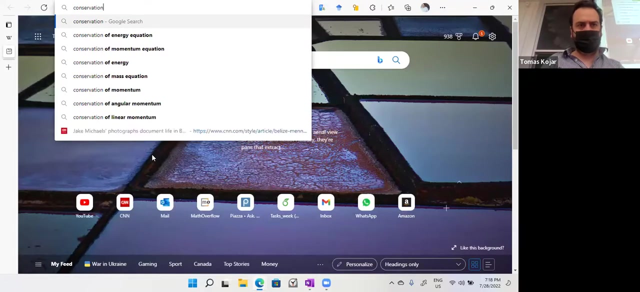 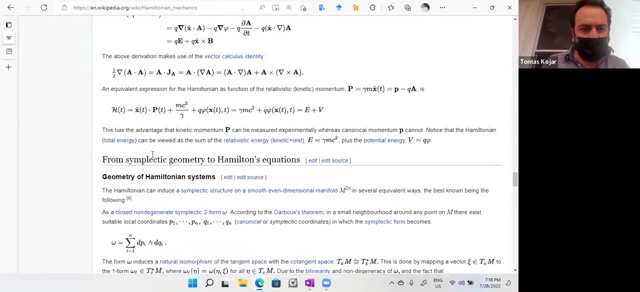 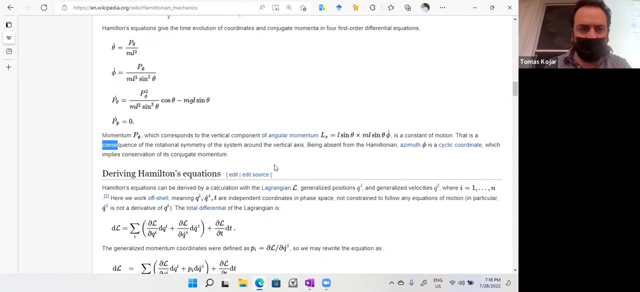 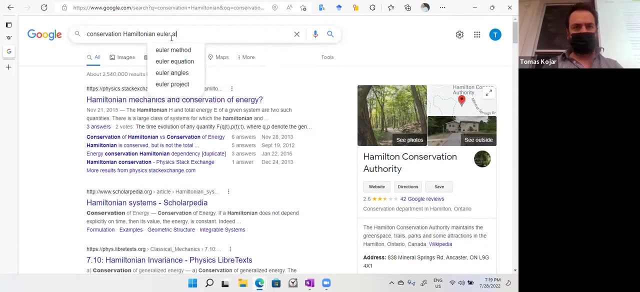 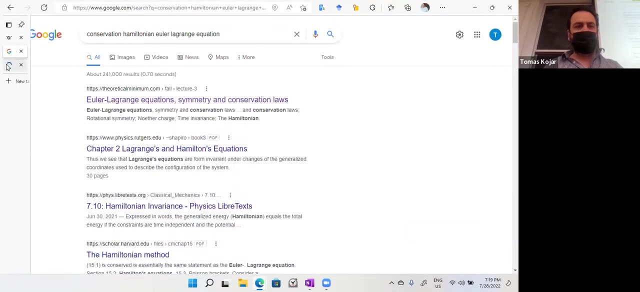 I remember there was Like- I mean, that's the one I talked to you about- Like for simple systems. it's just like kinetic plus. 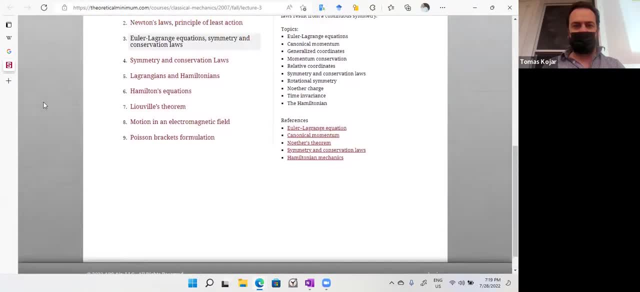 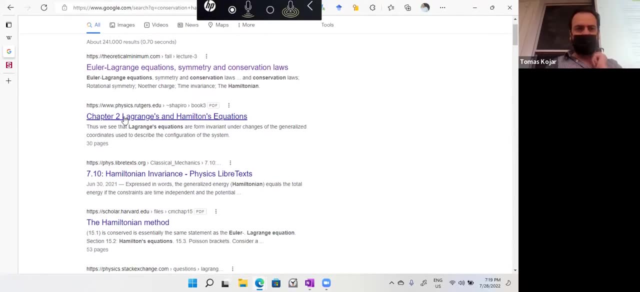 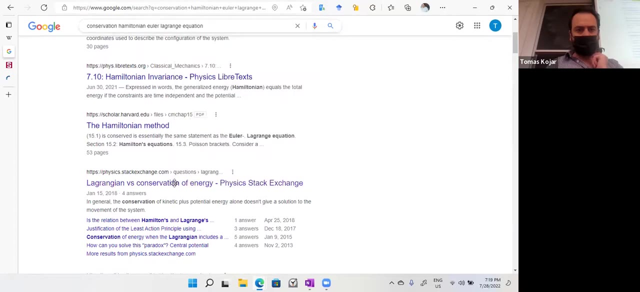 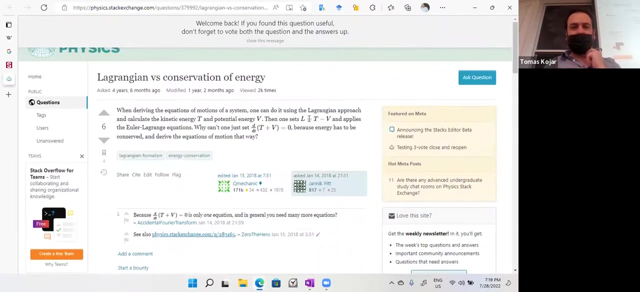 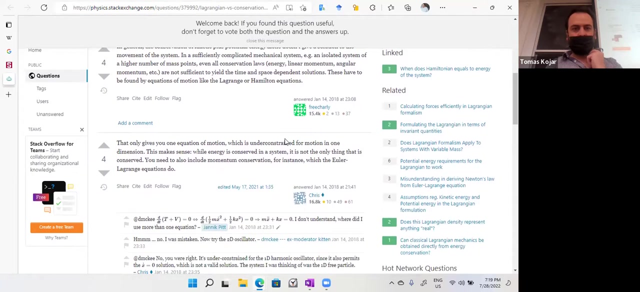 know that theorem? Have you heard about it? And that's how you get your. that's a different way to get. yeah, Euler Lagrange. I mean, you asked me what, why I was studying Lagrangian, And okay, yeah, this is the one you talked about, Right? Yes, So. 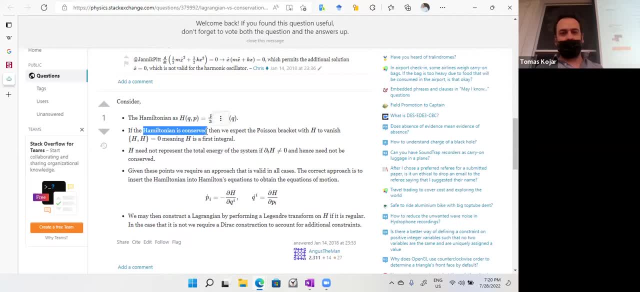 that's what I remember, that. So, yes, so that will be so if you have applied: Yeah, it's exactly the same thing. You take a variational derivative. If you look at the, I mean, I mean this is the stationary like, like, what is it? 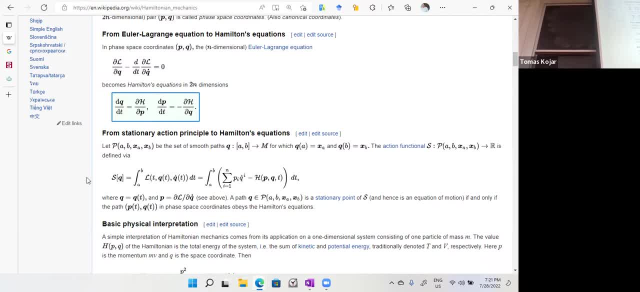 So, yeah, So you are going to do that. Huh, No, but you want to bring the solution to the Euler Lagrange And I want to write that here. Actually, I think we don't have to, maybe. Okay, that's all right. 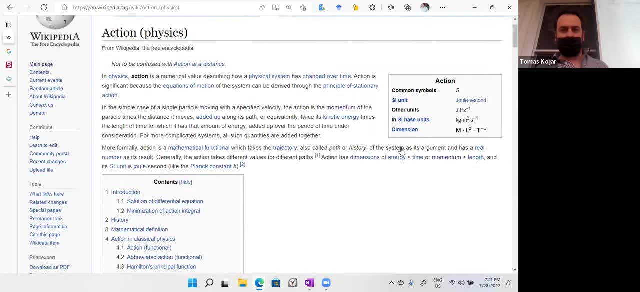 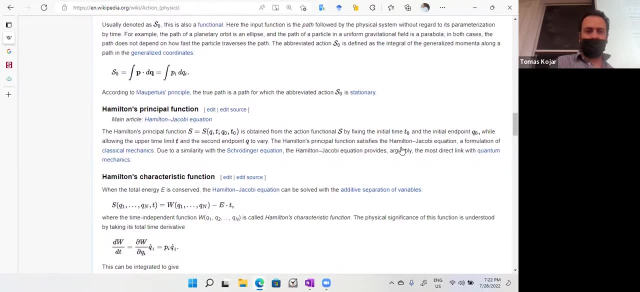 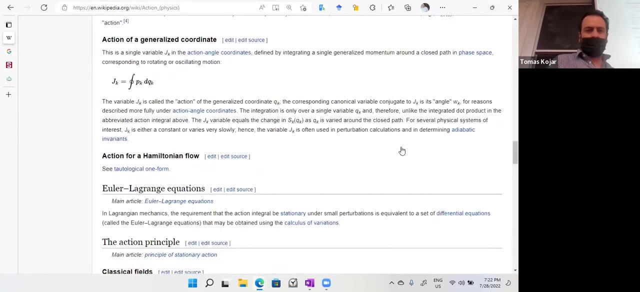 Sure, No, it's not pure math. Okay Fine, That's fine, All right, All right, I'm just going to use this one. Okay So, let's see, let's see, So, let's see. So, let's take the two sides. 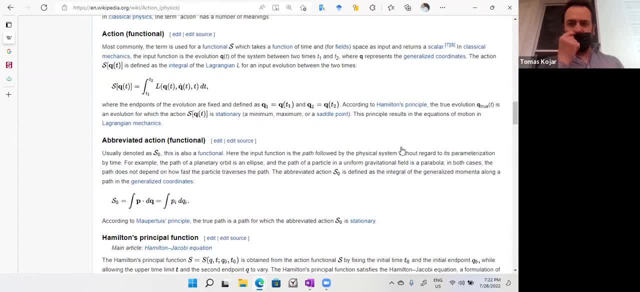 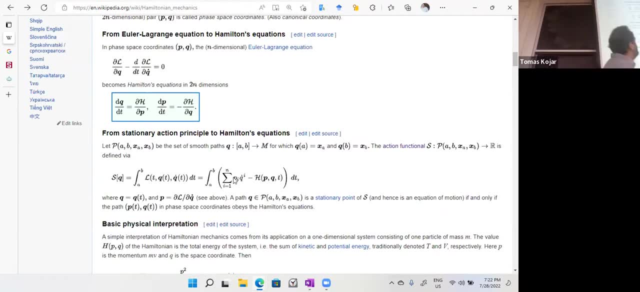 Let's say, let's take the random. It takes two sides And then you look for the right, So Lagrange. but I don't understand the thing they wrote here. There's a explanation: Momentum times, velocity. what is that? acceleration? 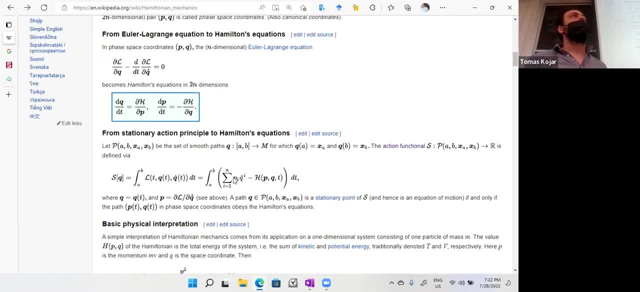 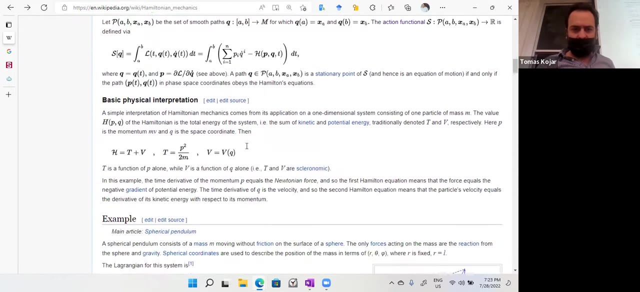 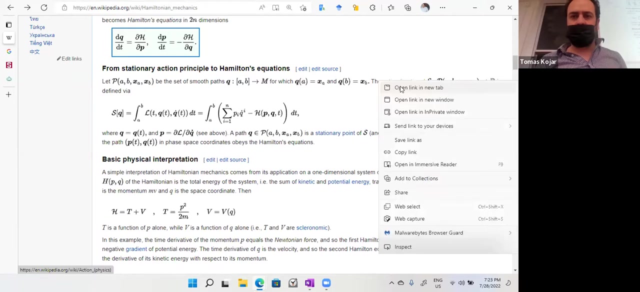 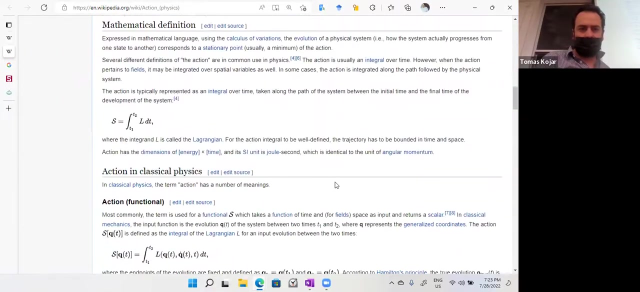 Like a Newton's law right Two times mv. Like how do they, why are they looking at like you say, why are they looking at this? Oh no, I want to know actually. Um, why is t minus v? 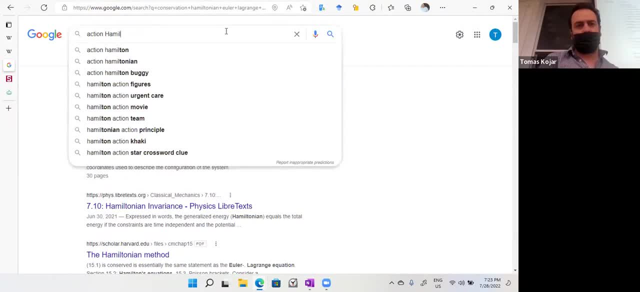 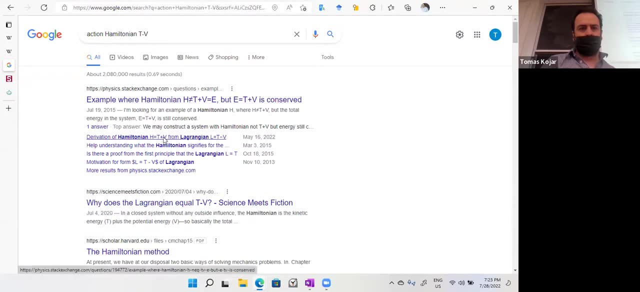 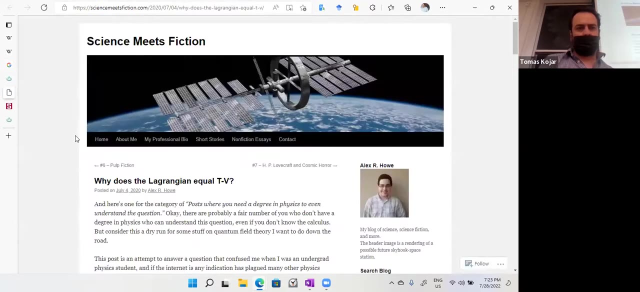 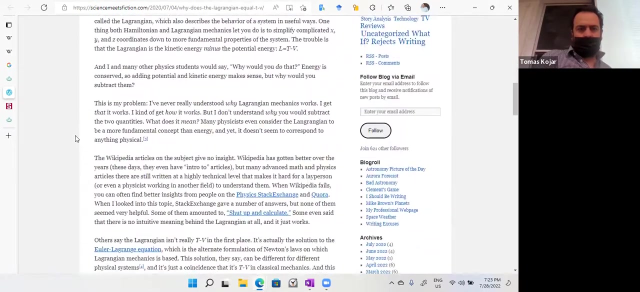 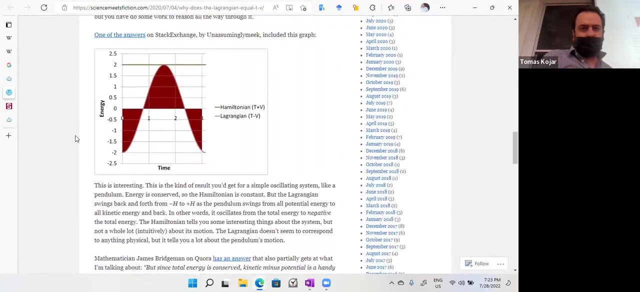 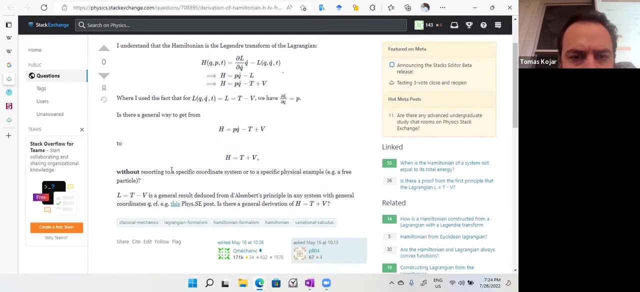 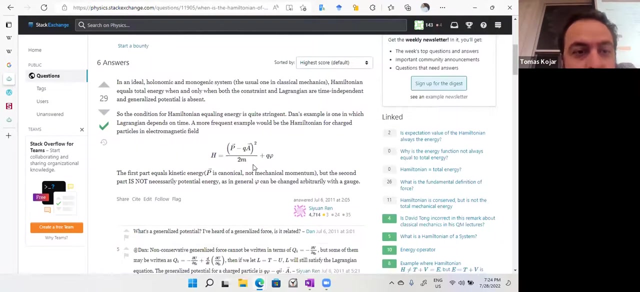 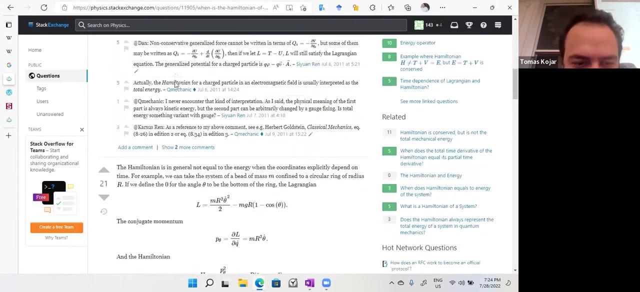 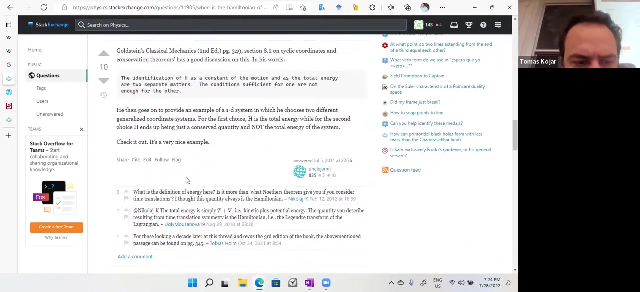 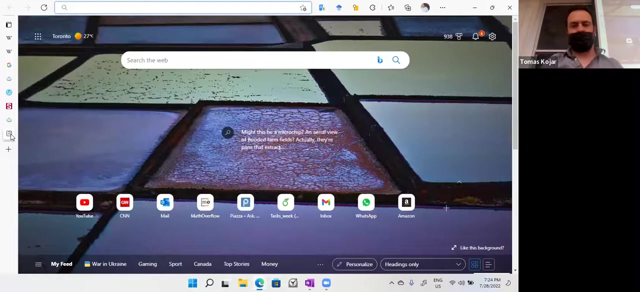 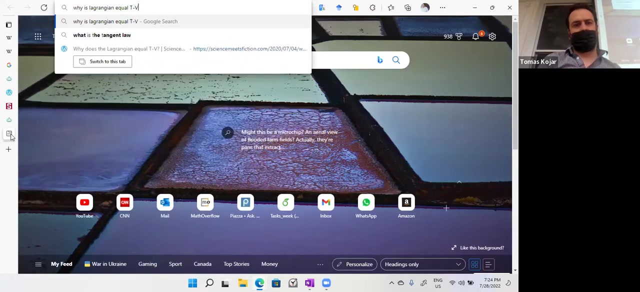 So why is it um? why is t minus v Yes? So why is this mathematical? Oh, we're actually going to do holonomic. You might get answered. Yeah, I mean here. yeah, we're doing very general stuff. 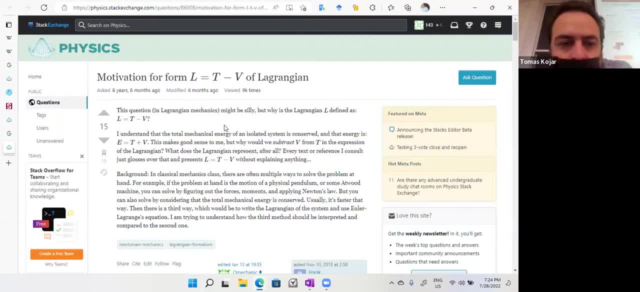 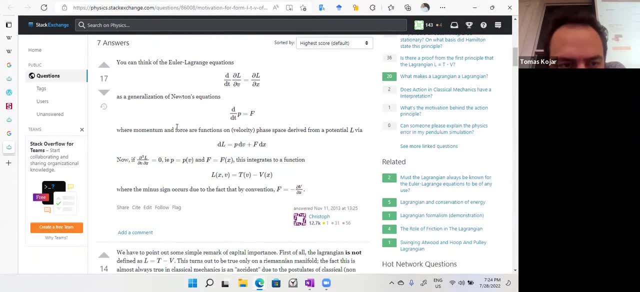 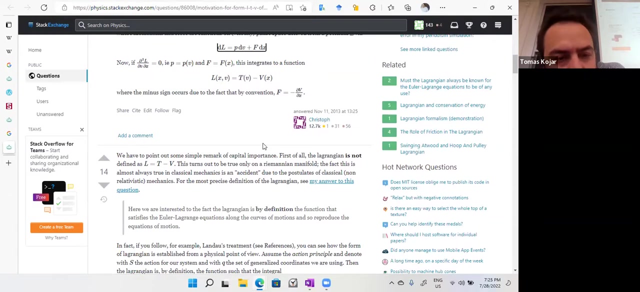 So I don't know, like the physical, I know mathematically why, but I don't know why. Okay, Again, I mean, this is the oh wow. But what would be the lambda? What would be the multiplier? 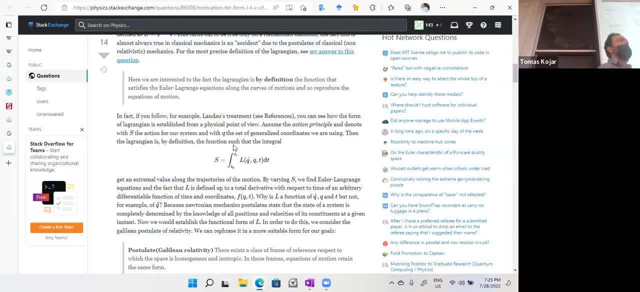 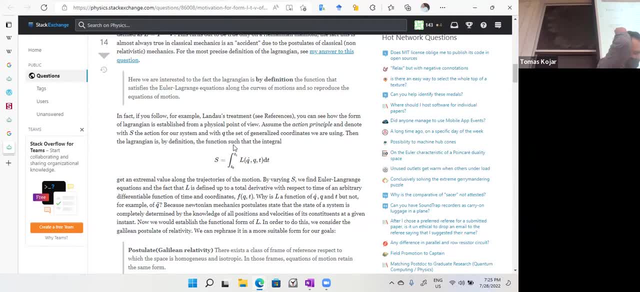 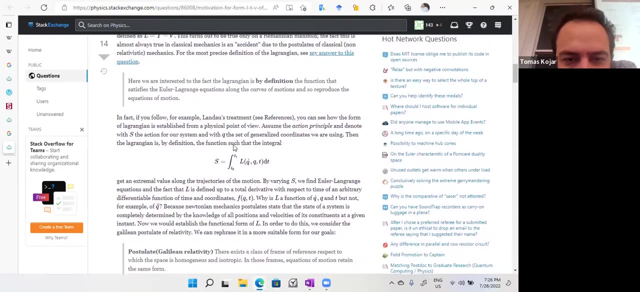 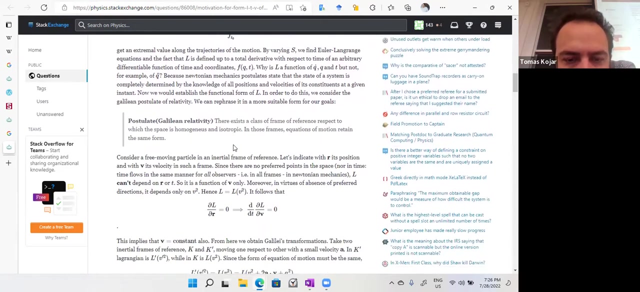 a, a, a, a, a, a minimize. Why is it lambda? Oh, the language is not. I know it's not that, but why does it turn out to be? Yes, You can only like one, then you get. 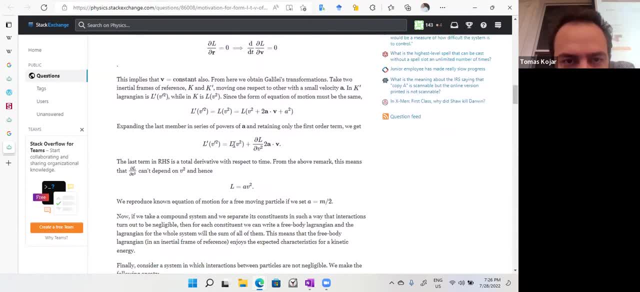 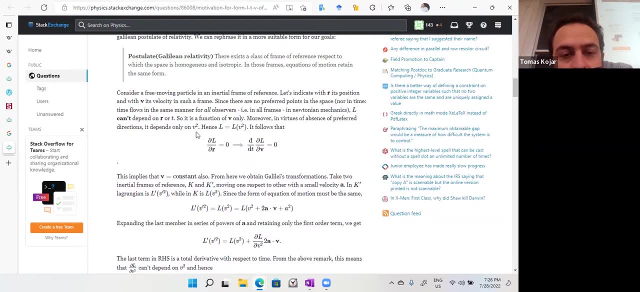 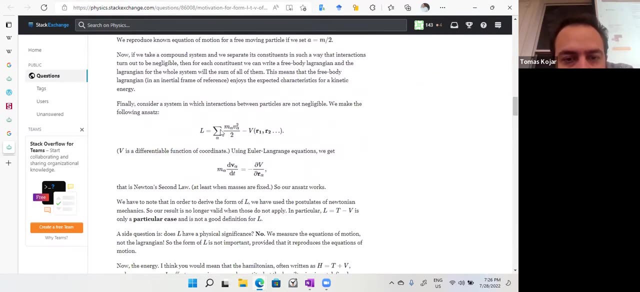 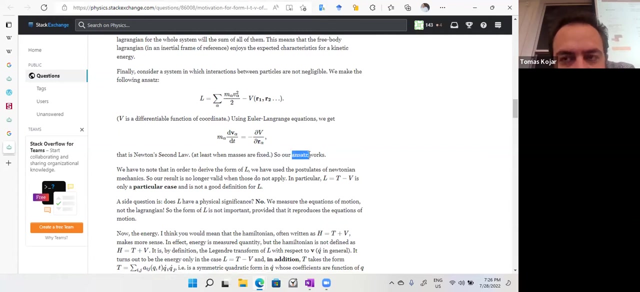 I mean, all these guys start from what we have, right: Ole Lagrange, right, You see? Like they start from Ole Lagrange and they prove that, that it's T minus V. But then when they say Ansazli, it means a guess, so they guessed it. 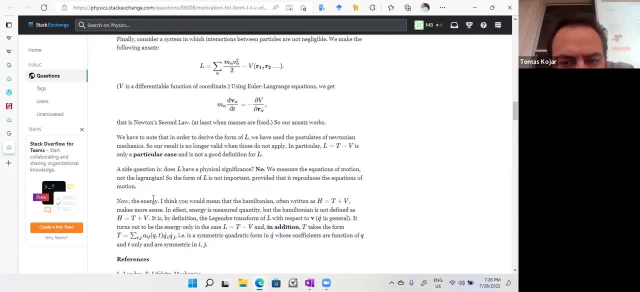 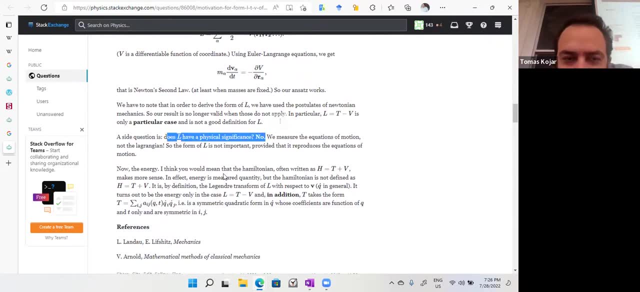 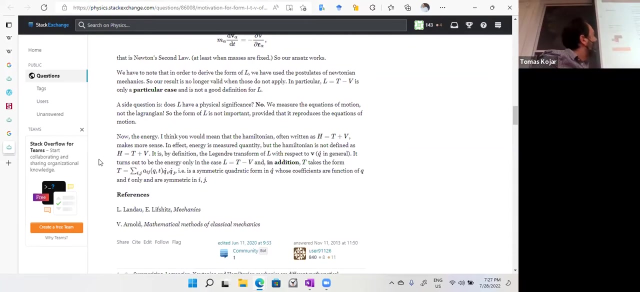 But how do they know? And it says it does not have physical significance. I didn't expect that. I thought it had some meaning Because I heard action all the time, Like if you read papers, people are very interested in the action. 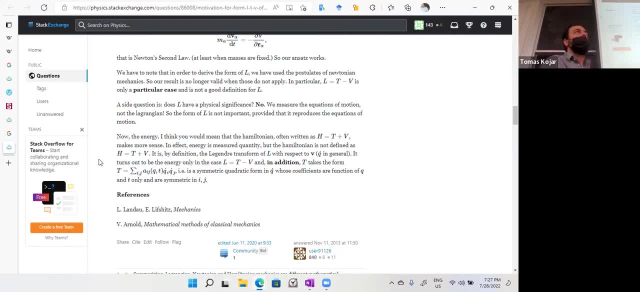 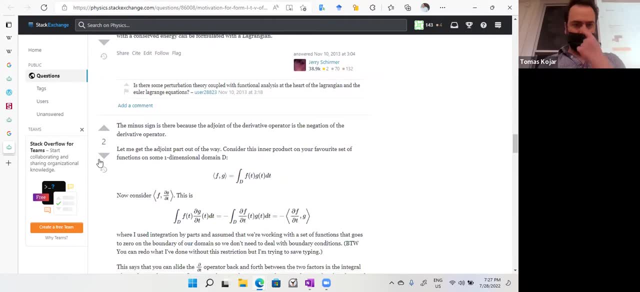 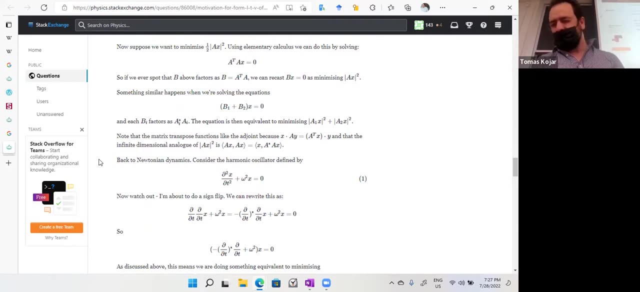 Like the action inside The integral? And you are, but you always start with the Hamiltonian And then No, no, it's the same action. But here your group is simpler. You just have vector space operation Because you have a function space. 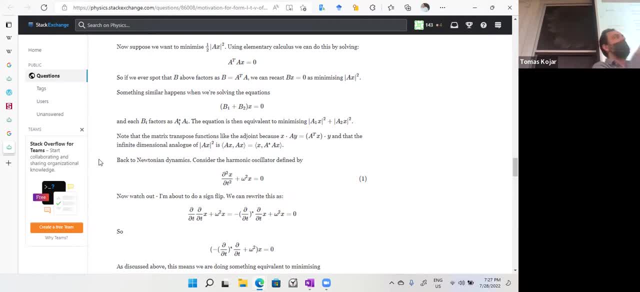 And adding two elements in the group gives you another element in the group. That's like the contradiction, right? Remember when you want to go from one element to the other. You know what I'm saying. In a group, right, You have like one element. 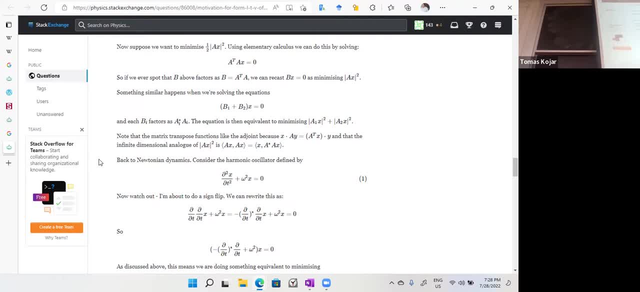 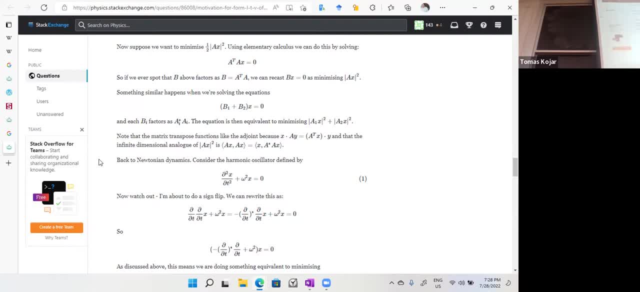 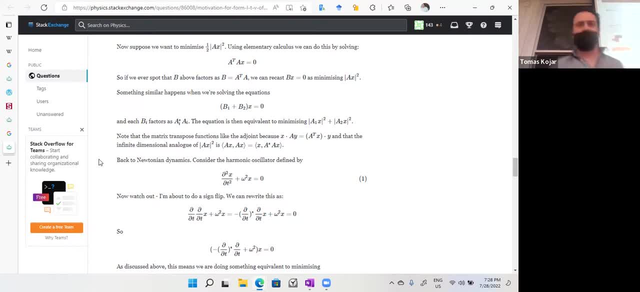 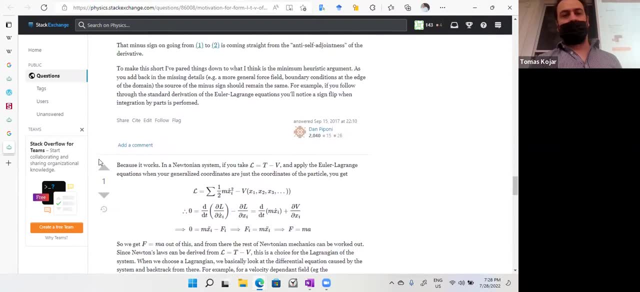 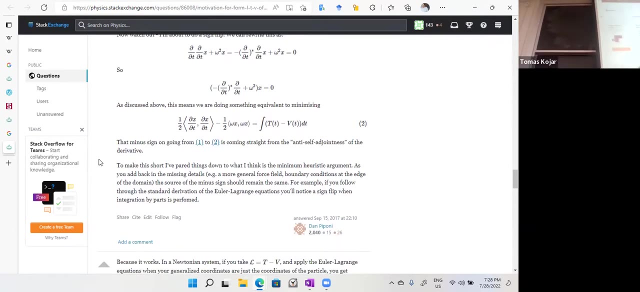 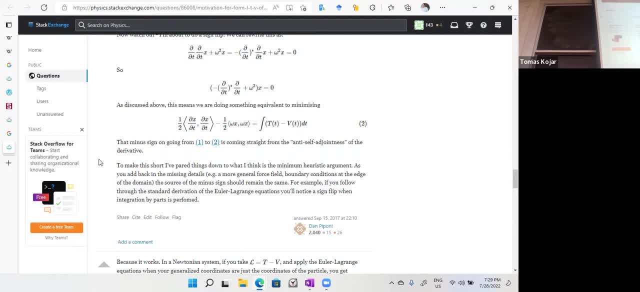 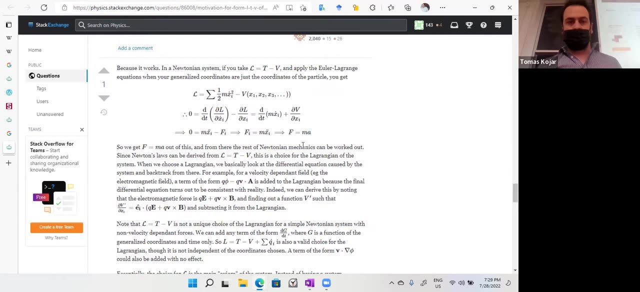 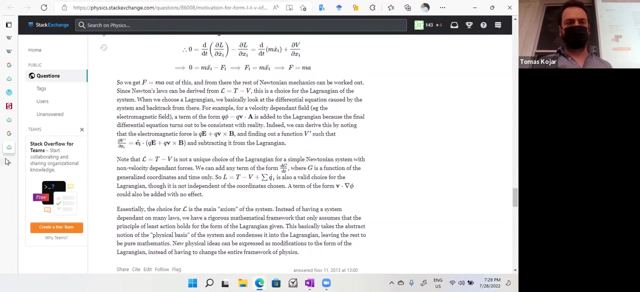 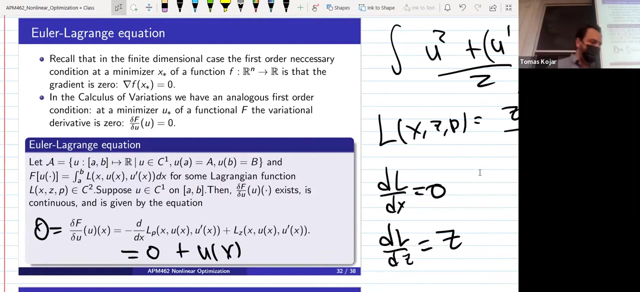 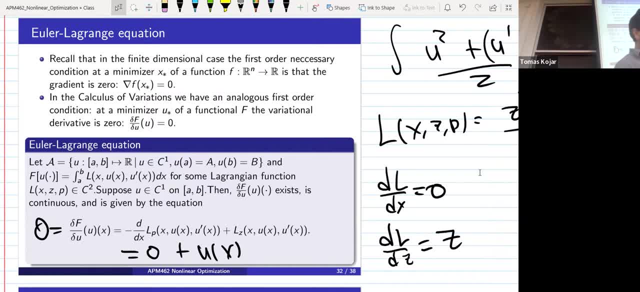 I didn't have time to read the whole thing. You were like: I'm like, I'm like, give me what You didn't have to like, send me a. but so what did you want? A record, never. 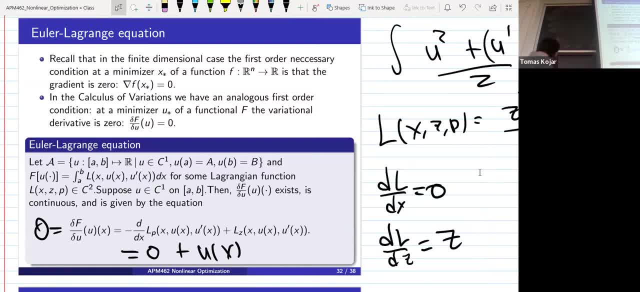 For what, Bill? Well, just for what? Yeah, well, I didn't see that. Yeah, I mean, I don't know. Yeah, I think it was a record. So yeah, I think it was a record. 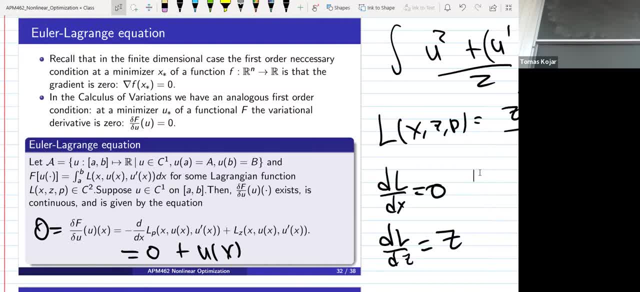 Yeah, And so, uh, I don't know. Yeah, I'm not sure if that's fair, I don't know, But I'll put it up on the on the page. Uh-huh, I don't know, Uh, but um. 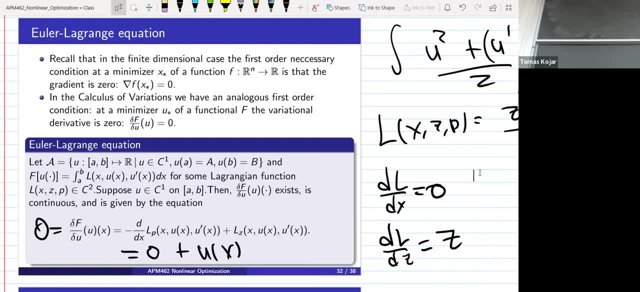 Yeah, You know it was. It was Good. I don't know It was um, I was Good. I'm going to look at that one. Yeah, Um, Oh yeah, Um. I'm sorry I can't hear you. 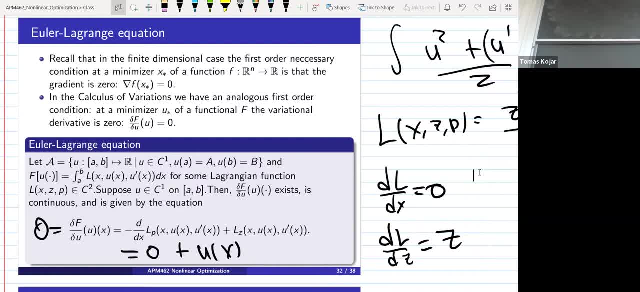 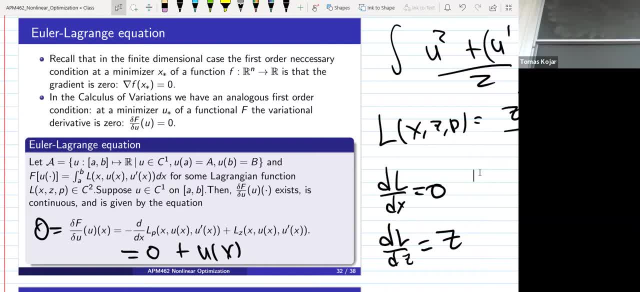 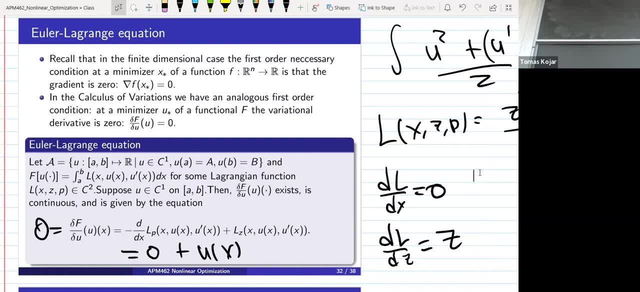 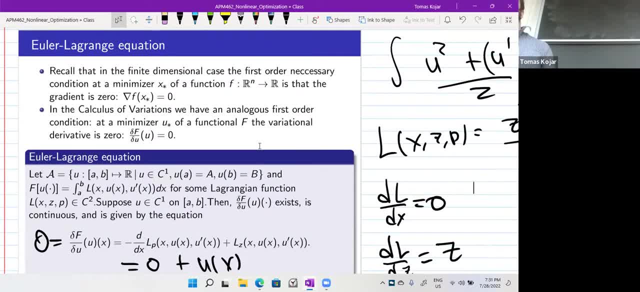 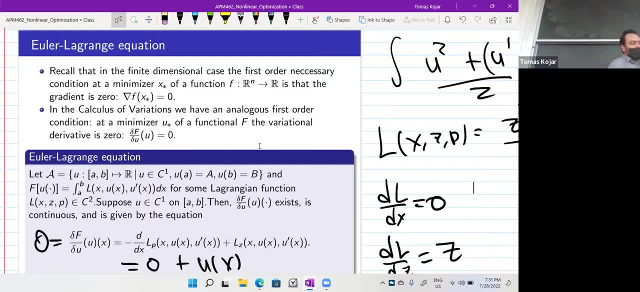 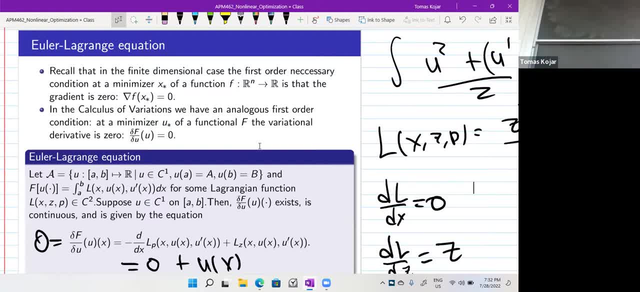 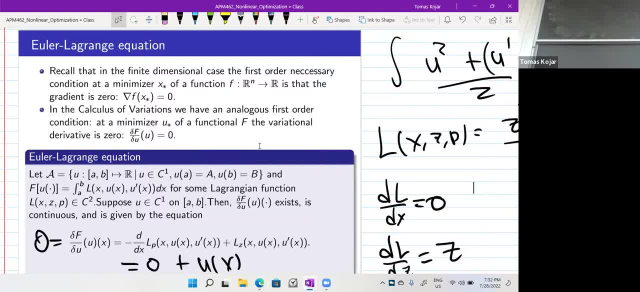 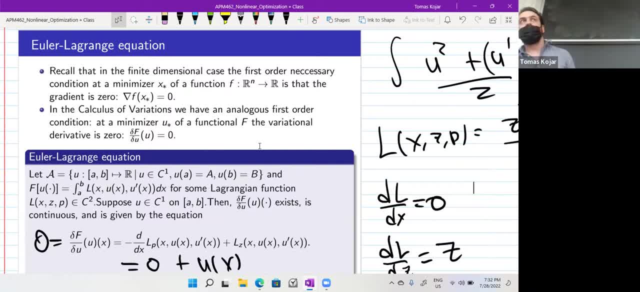 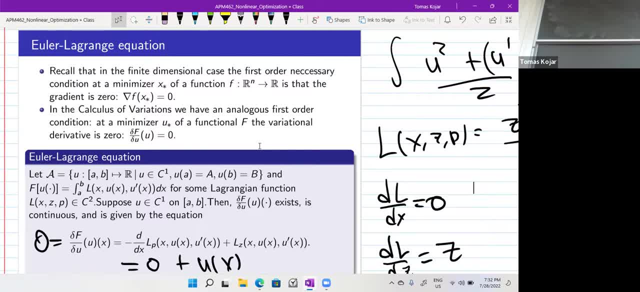 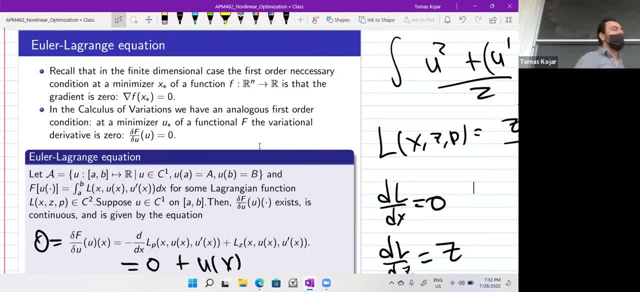 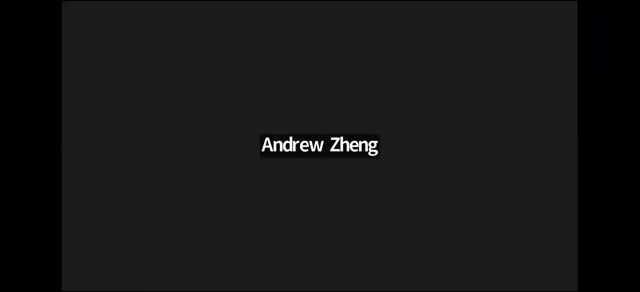